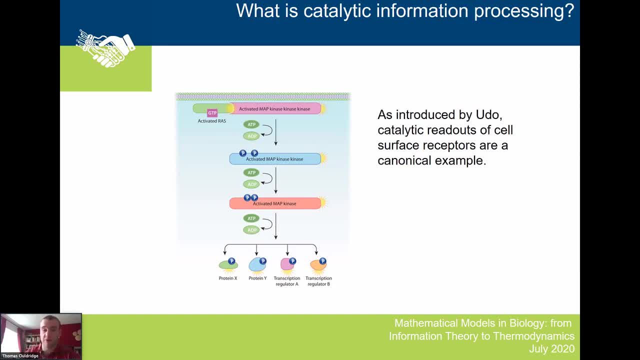 systems that read over those particles, And that's what I'm going to be talking about today. So I'm going to be talking about catalytic information processing systems and I'm going to be talking about catalytic out the state of those receptors and pass a signal on to the interior of the cell. um, can you see my? 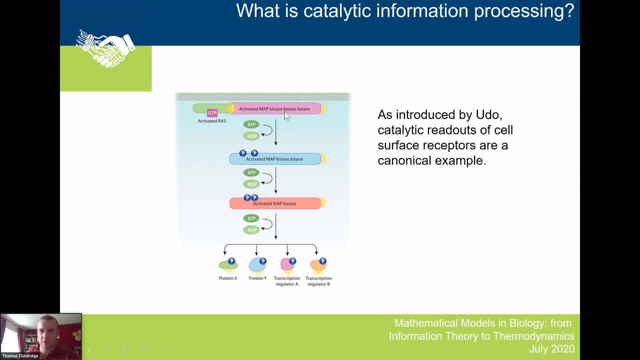 cursor, by the way. no, yes, the little white arrow. yes, i don't know if there's a way to make it better, but okay, let's, let's work with that for now. um, okay, so what happens in a canonical example is that um receptors that are anchored to the surface of a cell up here become activated by 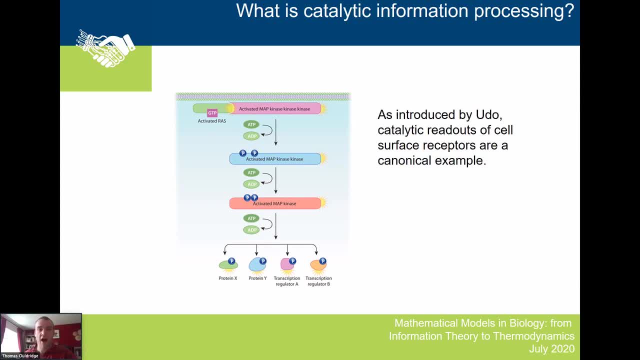 some process in the exterior and when they're activated they can act as catalysts to catalyze the conversion of downstream enzymes from an inactive to an active state, and those uh, those activated enzymes, then go on to catalyze uh enzymes further downstream and so on all the way potentially to 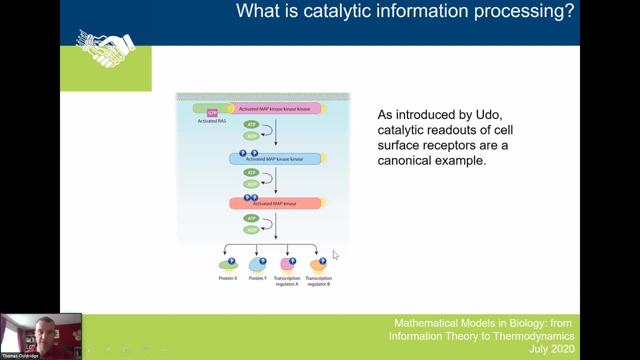 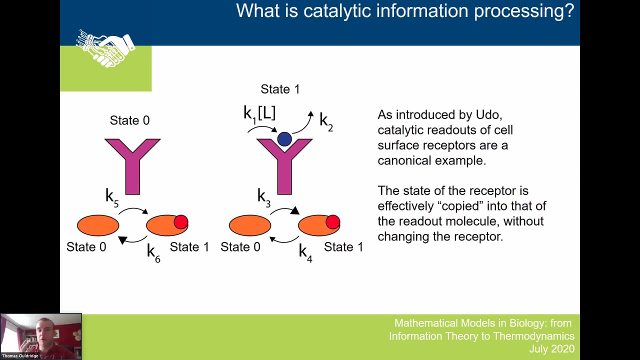 transcription factor regulation or whatever, whatever response the cell needs to have to the external signal. so, um the one, if we, if we really want to abstract what these things are doing, we can talk about them effectively copying the state of the receptor into a readout molecule. so this, this purple. 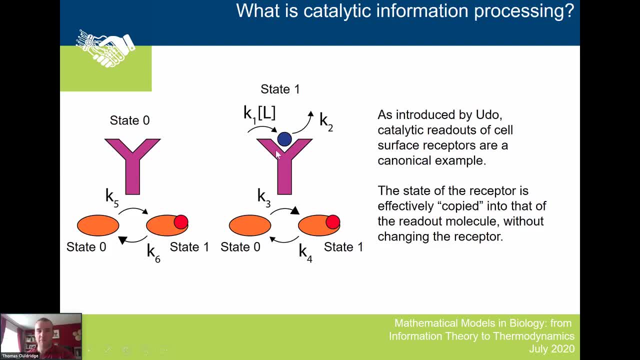 y is a receptor molecule. it combines to a ligand with a rate that's proportional to the concentration, which was very important in sarah's talk and um. the ligand can unbind to switch back to the other state. so we can call this state zero when there's nothing bound and state one when you, when you have. 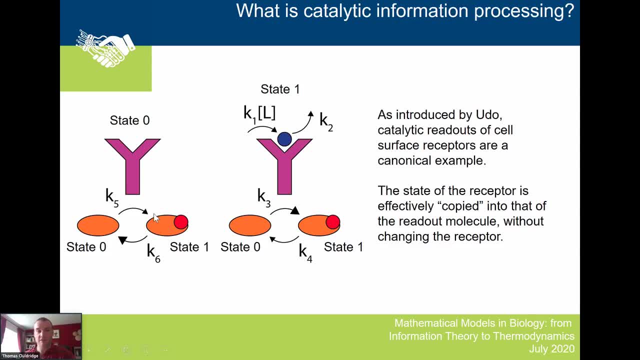 got a ligand bound. what the readout molecule does is when it's um, when the receptors in the inactive state or state zero, it can tend to catalyze the conversion of the readout from an active state, state one to an inactive state um, so typically, um some kind of dephosphorylation mechanism, the the readout. 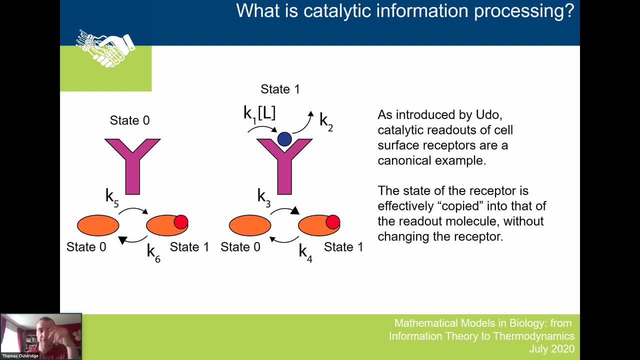 molecule can be converted from one state to another. when, instead, the receptor is bound to a ligand, the readout molecule can be converted from state zero to state one by the catalytic action of the receptor and therefore, if most of the receptors are in this state, if they're mostly bound to a ligand, 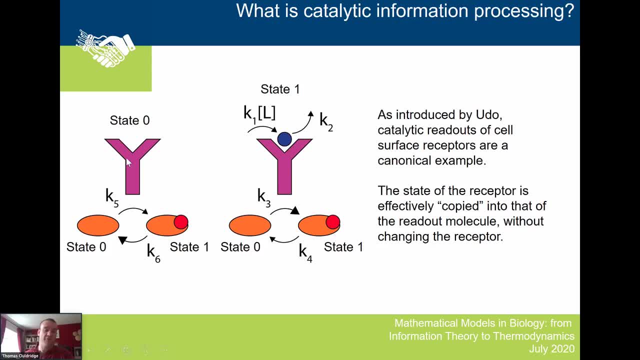 most of the readouts are going to end up in state one, and if most of the um receptors are in state zero, most of the readouts are going to end up in state zero. so here i've talked about specifically a bifunctional receptor that acts as a catalyst in one state to push the system in one direction. 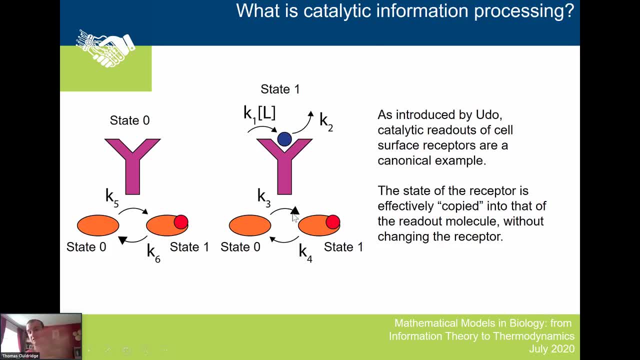 and a different catalyst in another state to push the system in another direction. that's a an idealization of how the system behaves, but broadly speaking, i don't think this story would be too unfamiliar to real molecular biologists. fundamentally, the important point here to note is i'm calling this thing a catalyst. why am i? 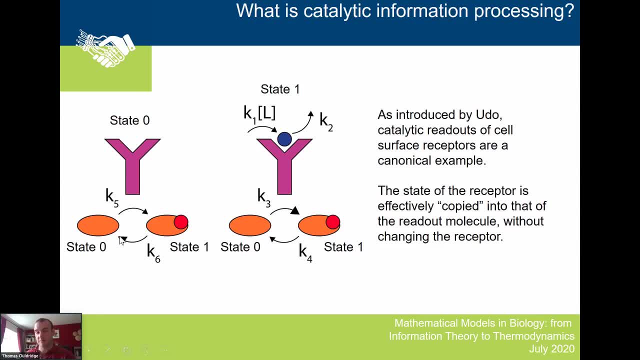 calling a catalyst. well, the state of the readout is being changed by these reactions facilitated by the receptor, but the state of the receptor itself is not changing. in the process, the receptor is accelerating reactions without being controlled in the receptor, and so the receptor is accelerating reactions without being controlled in the receptor, and so the receptor is accelerating reactions without being 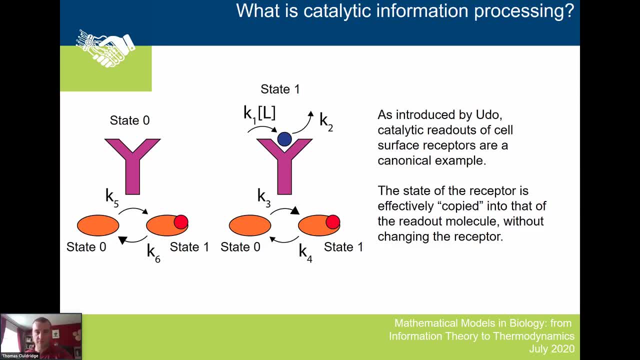 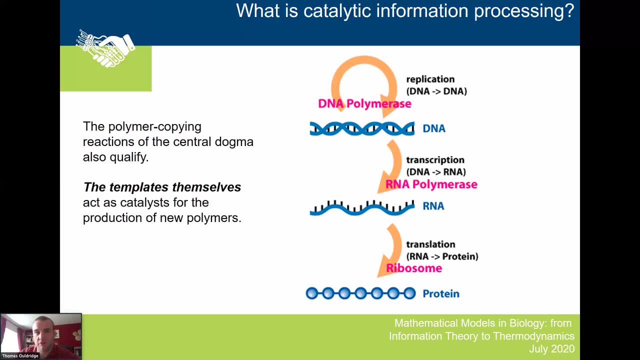 consumed, and that's why i'm calling it a catalyst. now, those are the most obvious examples of catalytic information processing, but they're not the only ones, and in fact, they're probably not the most important ones, and i would argue that the polymer copying mechanisms that underlie the central dogma of molecular biology are also. 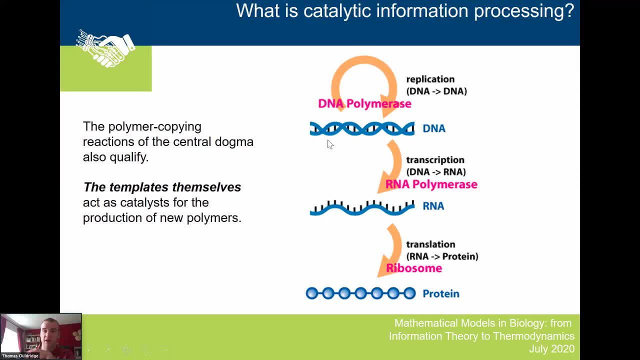 catalytic information processing. so what am i referring to here when i'm referring to dna templates, dna-double-strand being replicated into two double strands. i'm talking about uh dna being transcribed into rna and then the rna strand being translated into proteins and the fundamental. 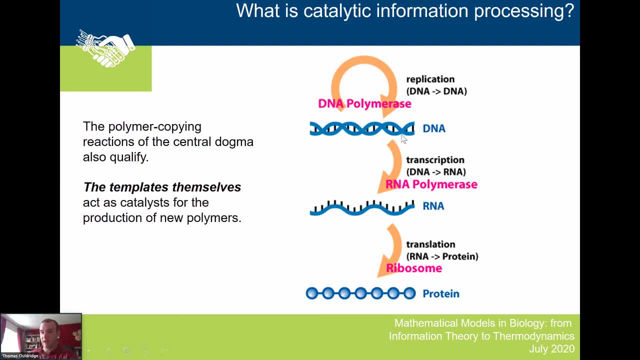 point here is that there's a specific sequence in the template dna, famous atgc base pairs. that sequence is preserved in the daughter dna when replication occurs, and it's also preserved in the RNA which is transcribed from DNA. and that sequence is also used to determine the sequence of amino acids in a protein, although not all of the information is. 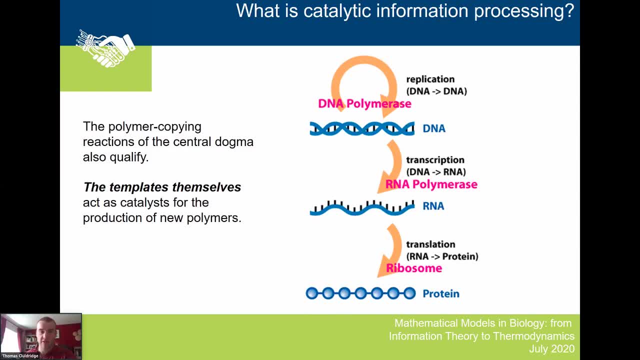 preserved. there's kind of a compression of information at this stage. Now, why am I calling this catalytic information processing? Well, at a very fundamental level, the templates themselves act as catalysts. In the absence of a DNA strand coding for a protein, you have a very, very slow 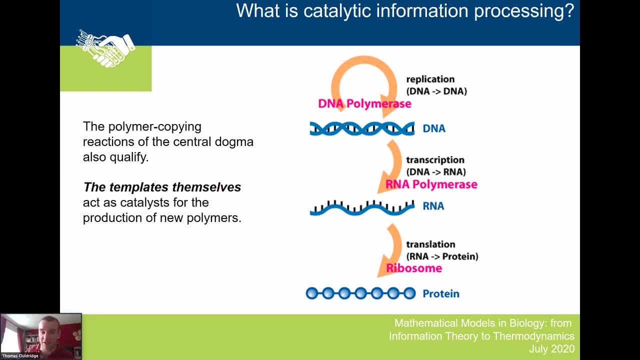 I would. we can approximate it as infinitely slow rate at which RNA, mRNA for that protein is produced, and an infinitely slow rate at which that protein is produced. You need the template there to for the reaction, for the production of the mRNA and the protein. Furthermore, at the end of the process, the template is recovered, The DNA that is used to make the mRNA. 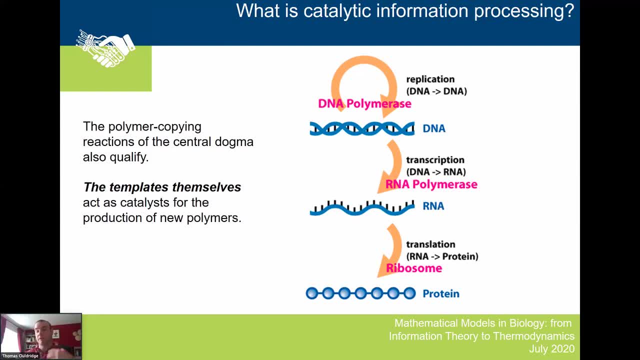 isn't destroyed by the process of making the mRNA. We get it back, and so it's contributing to the reaction. it's accelerating the reaction, but it's not being consumed. so, at a very fundamental level, it's a catalyst. So I've identified these two. 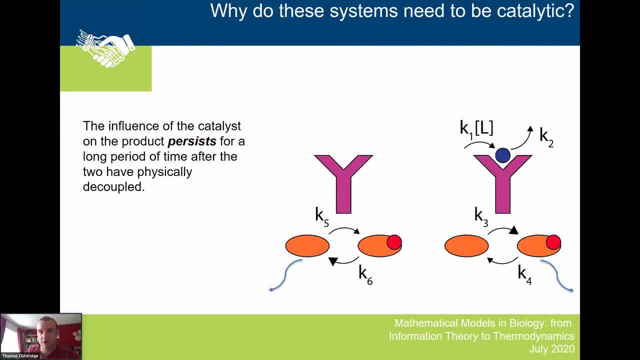 So I've identified these two important classes of information processing systems in biology and said that they're catalytic. Why is it important that they're catalytic? Well, the reason, I believe, is that if something acts catalytically, it means that the effect that it has on its, on the downstream product, can persist for a long period of time after the two are no longer bound to each other. 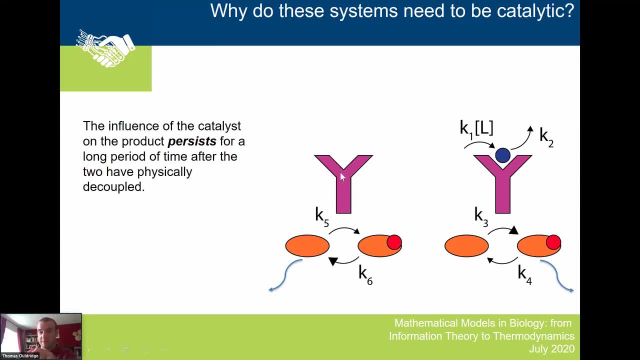 So in the particular example of the receptor that is catalyzing the conversion of a downstream readout, the receptor, when it's not bound to the ligand, catalyzes the readout being turned off. that readout then diffuses away in the off state and it stays in the off state. 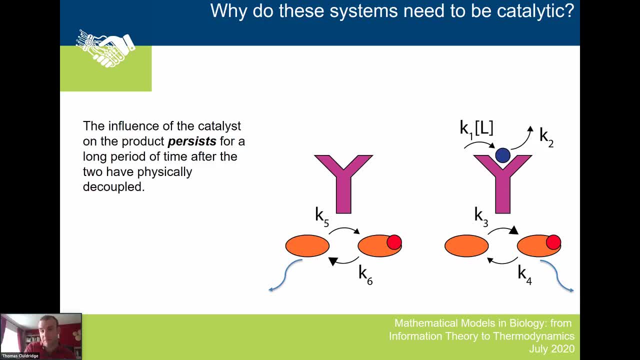 It doesn't need to stay bound to the receptor for it to be kept in the off state. Yes, We have a question from the audience. I hope I'm reading this correctly. If it's really a catalyst, it should enhance the backward rate, which is RNA degrading as well, right? 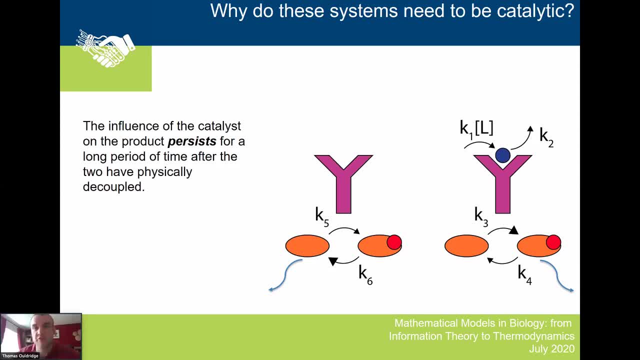 That's the question. Yes, it does, but it's driven so hard forwards that you never see that happening. The RNA degradation- I mean this- I'm going to get into the thermodynamics of these things in a moment- But the RNA template, in principle, if you are able to wind down the 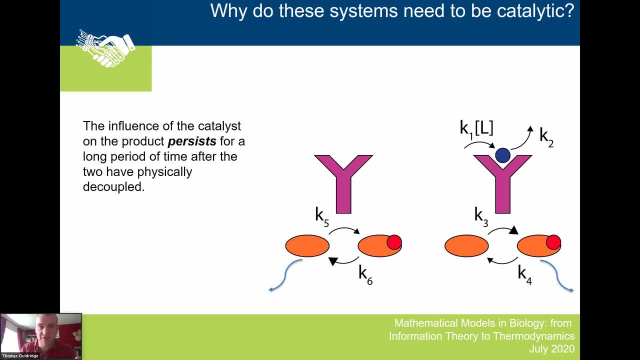 um, nucleotides, triphosphate concentration. in principle, the template could come back to the um, uh, the the product should be able to come back to the template and be disassembled there. now, that's not what happens in a cell. what a cell does is it has um, the reaction to produce. 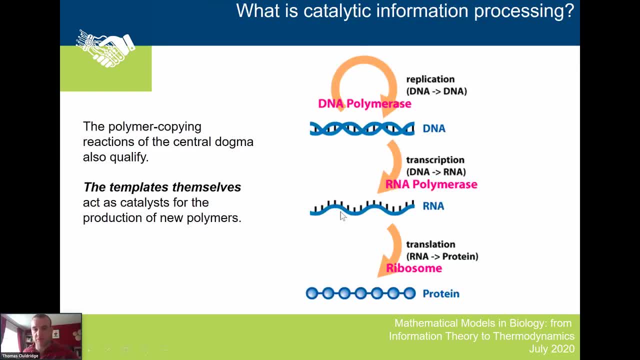 the reaction to produce the mrna, which is being strongly pumped with um free energy supply. basically, so it. so it overwhelmingly goes forwards. you never see it go backwards. and then they also have the degradation of the rna via another pathway, um which again is is driven with um free 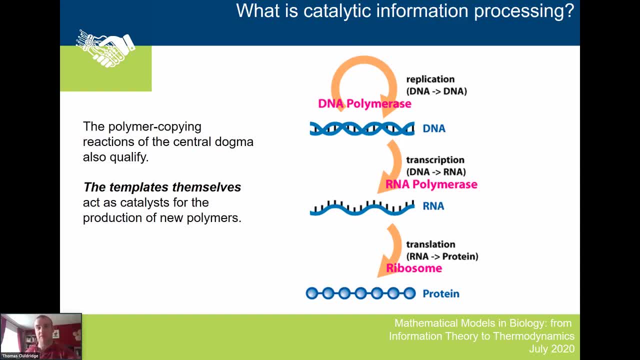 energy, and so you never see that one going backwards either. but in principle, if you, if you turn knobs of these free energetic driving towards zero, you would see these processes going backwards and forwards via the catalyst, and to some extent that's what i want to do in my experiments. that 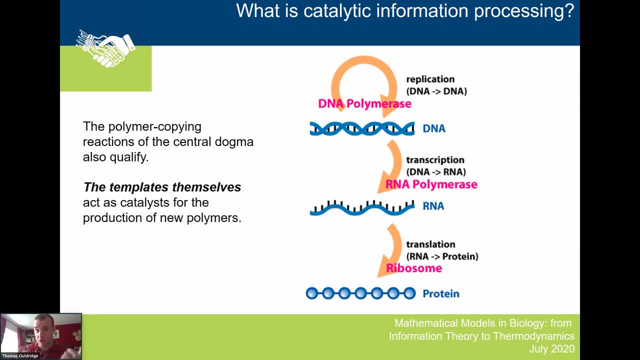 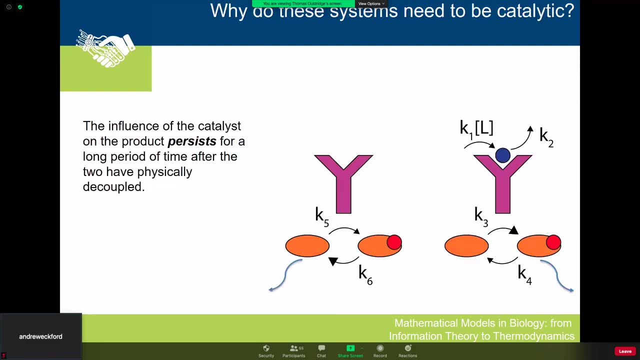 i'll get to later- is really actually reach these limits where you could could do that? does that answer the question? uh, the answer sounded good to me. um, i don't see a response from the question. asker, yeah, yeah, he says yes, thanks, great, okay, so, okay, so. so what i'm saying is that the, the catalytic action, um, allows the, um, the product. 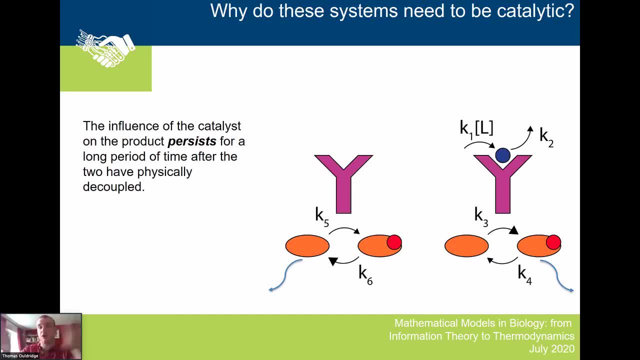 and the substrate to go their separate way, the product and the catalyst to go their separate ways after the interaction, but retain the, the change that was made. now, this you don't get in the other model of um signaling, um signal transduction in um molecular systems, which is 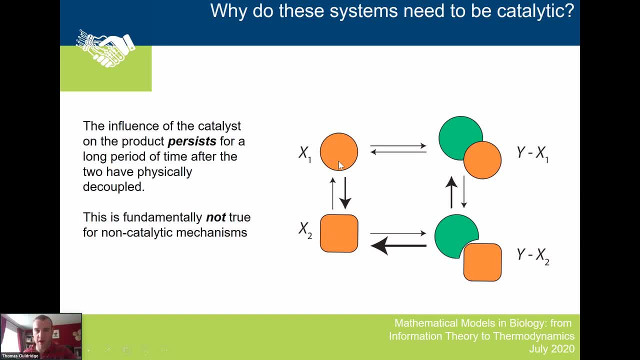 the моей eric binding. so if i imagined my x here, a two which can switch between two states, is my downstream molecule and my upstream is this green uh protein, say, and when the green protein binds to the, the orange one, it tends to favor converting it into this. 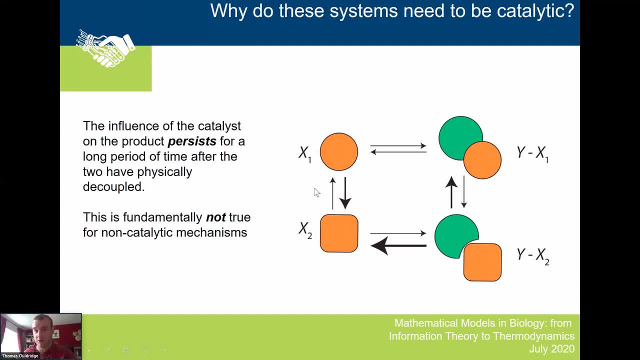 circular state, rather than the square state that udo was talking about in his talk, and um when and and cells do indeed use this. however, as soon as the um uh, as soon as the, the green upstream uh protein unbinds from the um downstream, one, lets it go again, it will then immediately convert back to its um unbound state. it turns 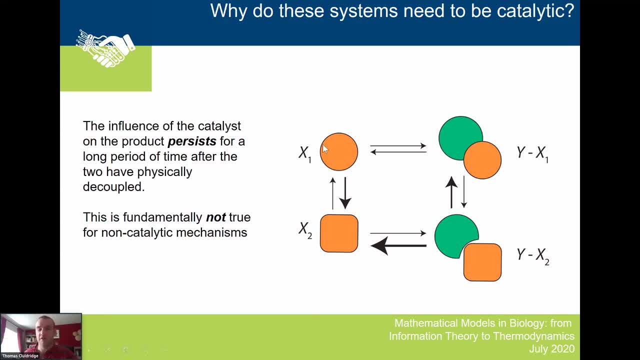 out that you can do the analysis and in order for, if you wanted the downstream protein to to remember the influence of the upstream one from the past, you'd necessarily be violating the second law of thermodynamics. you'd be creating time asymmetries without an input of fuel, and that's um, that's a. 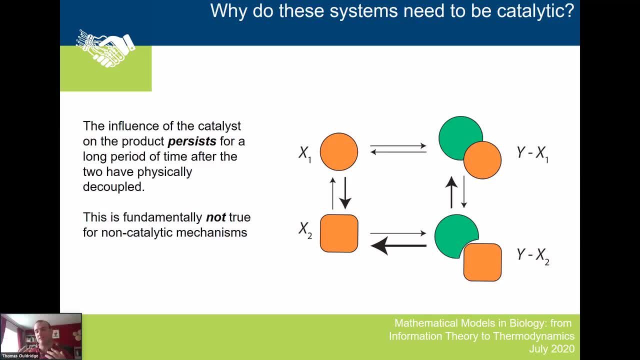 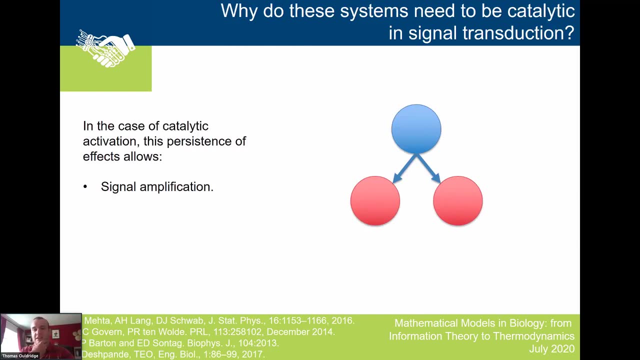 violation of the second law. so you don't get this ability to um persistently modify your downstream product unless you're- unless you're- acting catalytically and consuming fuel. okay, so so why? why is this catalytic um action, uh, particularly useful? uh, and with what we've hinted at, is that indeed it. 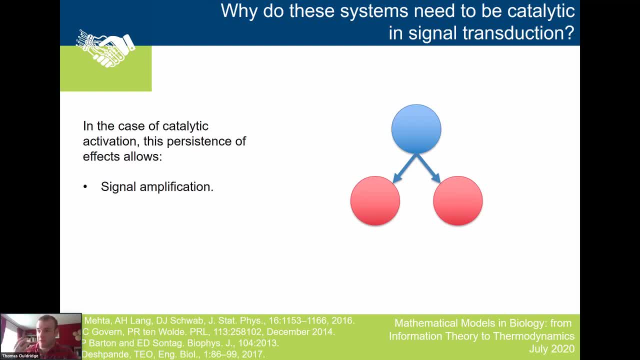 there's a cost to it, which is that you need to consume um a supply of free energy to signal in that way, um, so it better have some important uses. well, given that the product can uh detach from the catalyst and they can go off and have an independent existence from each other. what that means is: 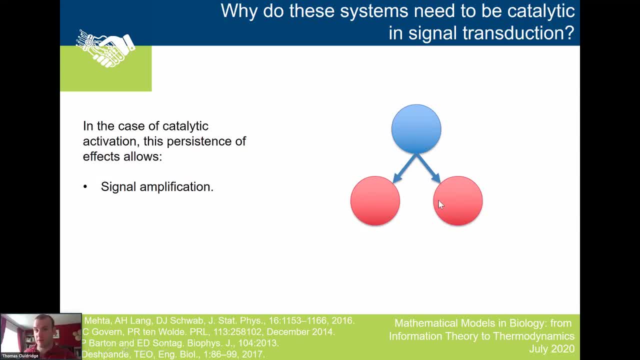 that one upstream molecule can activate two downstream ones, or three or four, or indeed an arbitrarily large number. so what that gives you in these signaling cascades that i talked about at the start is the potential for extremely strong signal amplification. a single um input speech, you can activate a whole host of downstream ones and on a similar level. there's no reason why the 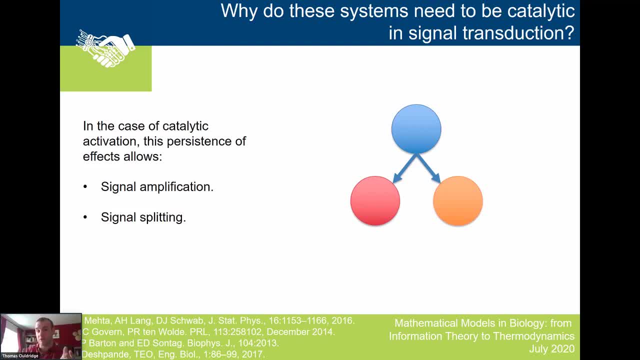 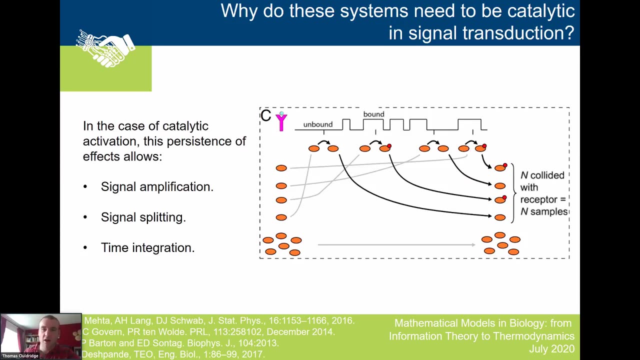 downstream things that you need to interact with have to be the same. they could be different from each other, and that gives you the option of uh splitting your signal without um, without corrupting it essentially um. my collaborator, peter rhine, um argued very eloquently that another important use. 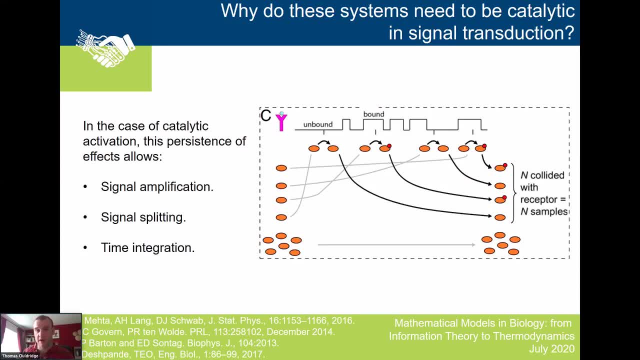 of of this um persistent modification, uh mechanism is that it allows you to do a time integration, so um the classic burr purcell story that was touched upon um on the first day, is that um a single receptor which goes from being unbound or bound to a ligand molecule at any one time. it 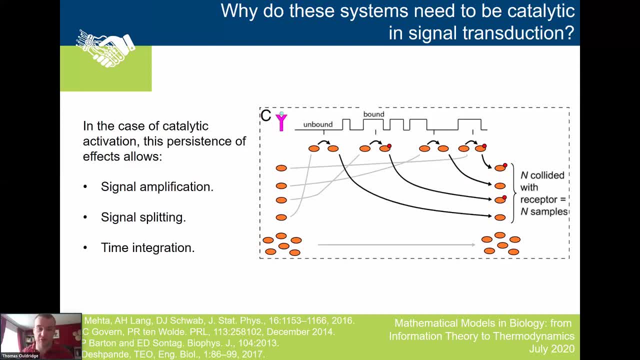 gives you an incredibly noisy reading of what's the concentration of the ligand in the outside world. however, if you're able to average that signal over time, you get a much more accurate guess at what the concentration is. but in order to average you need to remember the past. you need some kind of memory that that records what the 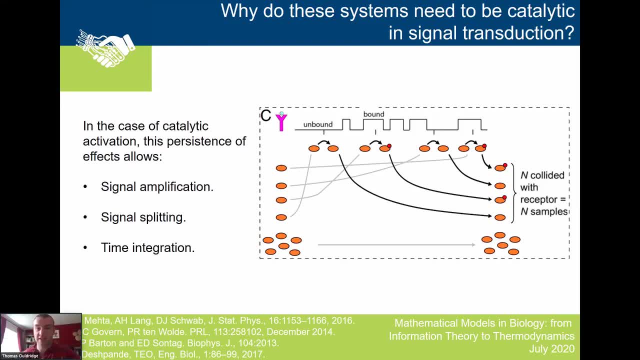 state was historically and the um. that's exactly what you get with these catalytic modification schemes, because the um, the upstream uh receptor, can catalytically set a memory and then that memory holds that state in principle for a long period of time, even as the catalyst is. 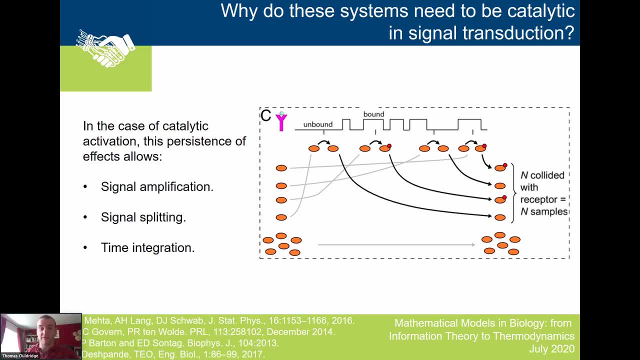 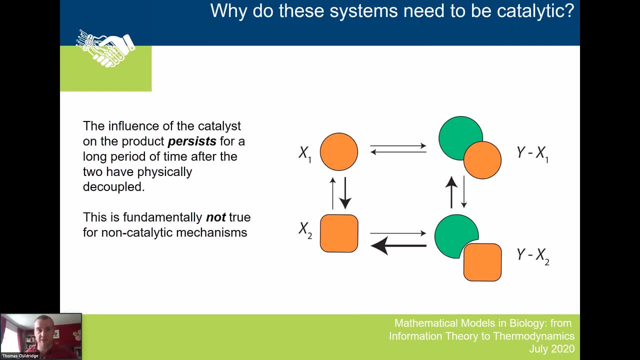 flipping around between the banks of the system and the system is going to have a long-term effect as a result in the unbound state And hopefully it's reasonably clear that you can't do this mechanism with this equilibrium binding mechanism. Finally, another thing it allows you to do: 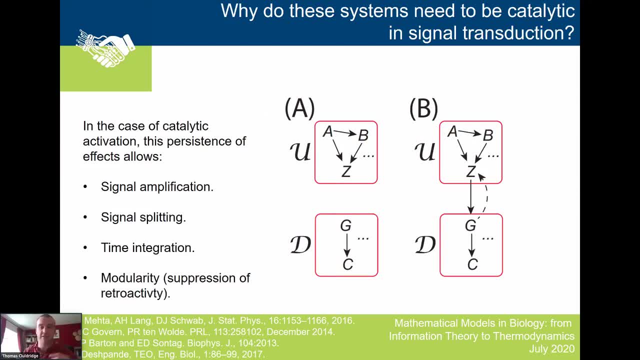 is if your mechanism for activating the downstream substrate is to transiently interact with it, turn it on and then diffuse away and not interact with it again. that means that the effect of the downstream substrate on you is quite small. In electrical engineering it's very useful. 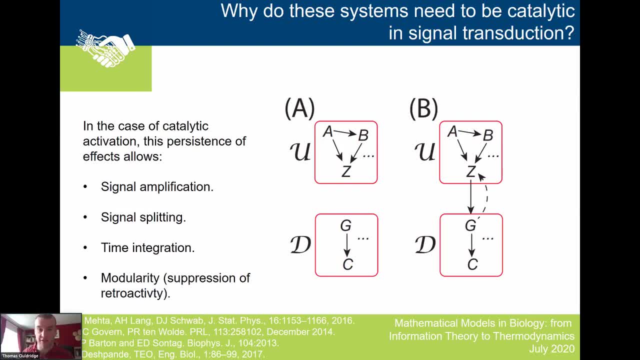 if we're able to make assumptions about modularities of circuits, If we can design one part of a circuit and another part of a circuit, an upstream and a downstream part, plug them together and have as little as possible feedback from the downstream subject to the upstream one. Once you start getting this, 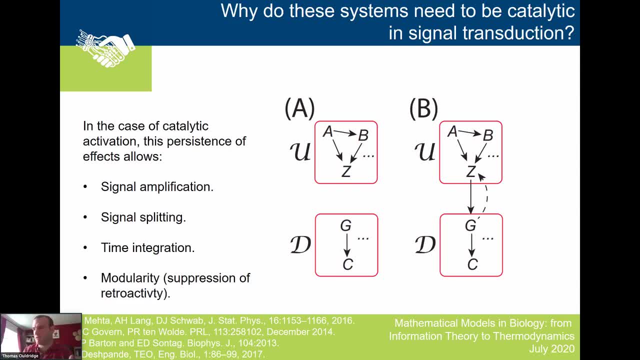 feedback or retroactivity, it becomes really, really hard to rationally design circuits that work the way you want them to. You lose this ability to think modularly And this catalytic activation, because you can activate the downstream module and then you only need to be interacting with it transiently. it gives you the opportunity. 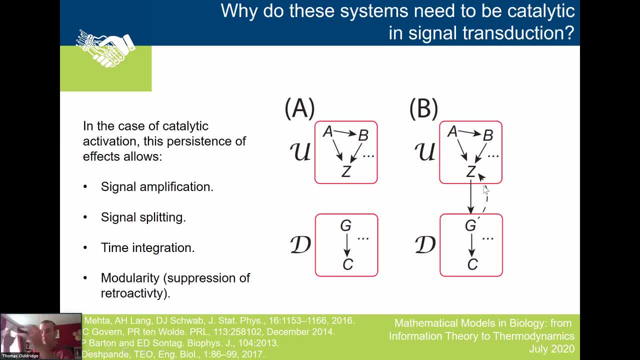 to really reduce this back action from the thing you're interacting with. You don't spend your time bound to it, sequestered for long periods of time, and therefore the retroactivity is small and your modularity is potentially quite high. So there's lots of uses for catalytic action. 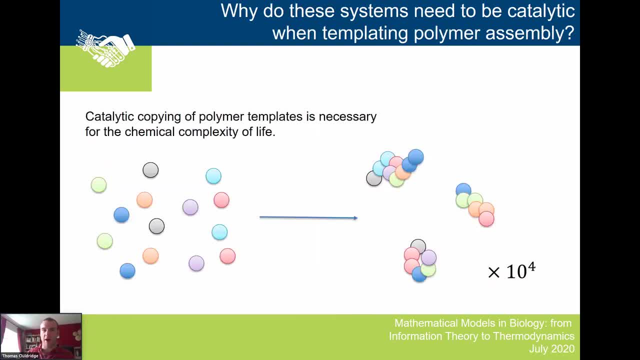 in signaling. What about the other example I gave, which were these sort of polymer copying mechanisms that I talked about in the central dogma? Just a moment, Thomas. We have a question from the audience. Is it true that integration of the signal will happen only when the catalysis is coupled to free? 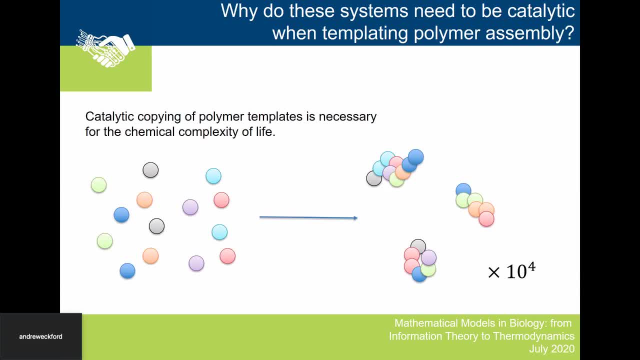 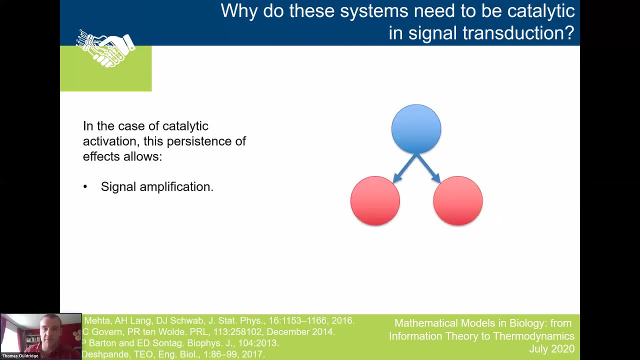 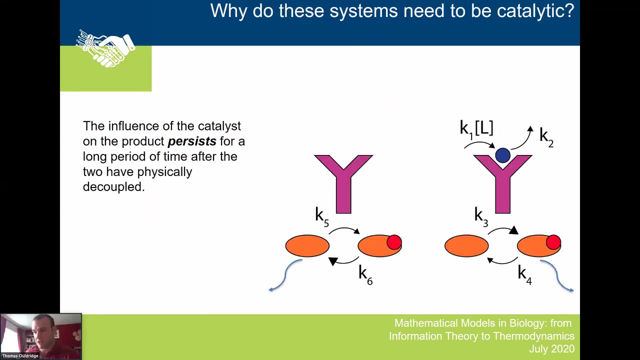 energy dissipation. If the catalyst only changes rates of the downstream reaction, say phosphorylation, would the downstream molecule be able to integrate. So you can, A catalyst can only, If I go back to this picture here. so the only thing a catalyst can do, as was pointed out, 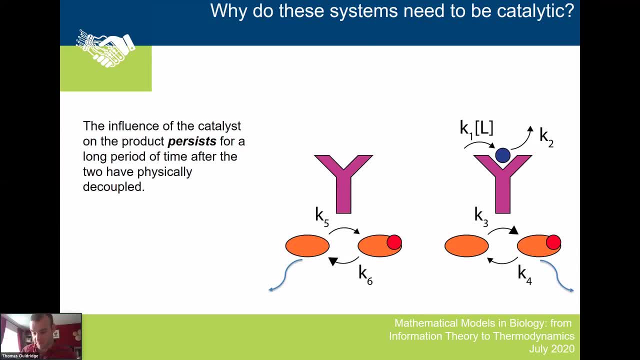 is accelerate both forwards and backwards processes in the reaction. The way these phosphatase kinase networks work is that the phosphorylation pathway is A phosphate group is taken from ATP and added to the downstream protein, And what the phosphorylation does is accelerate both, doing that forwards and doing that backwards, So both adding a phosphate. 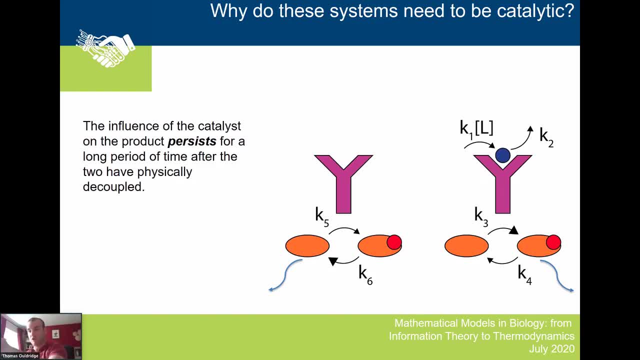 from ATP to your readout and removing that phosphate and giving it back to ATP. However, that's not the only way to switch between those two activation states. The other way to switch between those two activation states is just to release the phosphate into solution or get it. 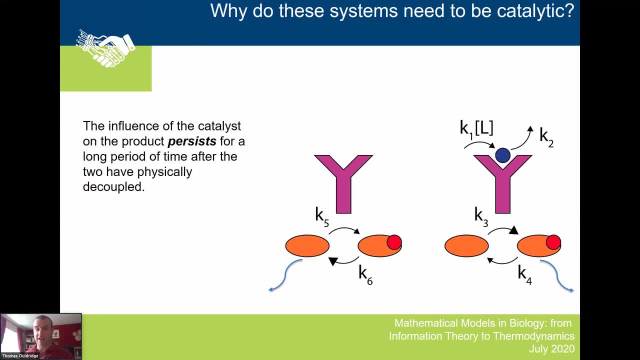 directly from solution. So the phosphatase accelerates the interchange of phosphate with solution and the kinase accelerates the interchange of phosphate with ATP And both of those process. One of those processes is downstream in one direction and one of them is downstream in the other direction. because when you go around in a 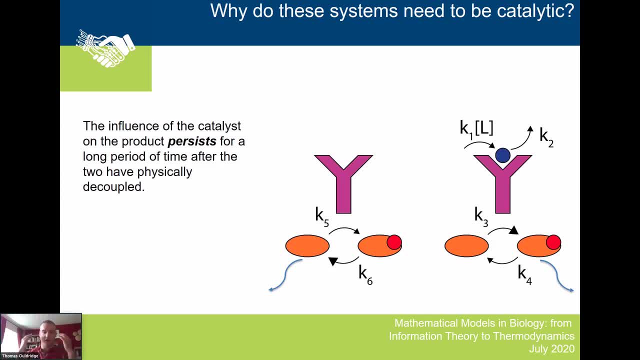 full cycle, you've hydrolyzed an ATP which is incredibly favorable, free energetically. So the presence of the kinase, what it does for you is it really ramps up both of these reactions, both the forwards and backwards reactions associated with taking an ATP. 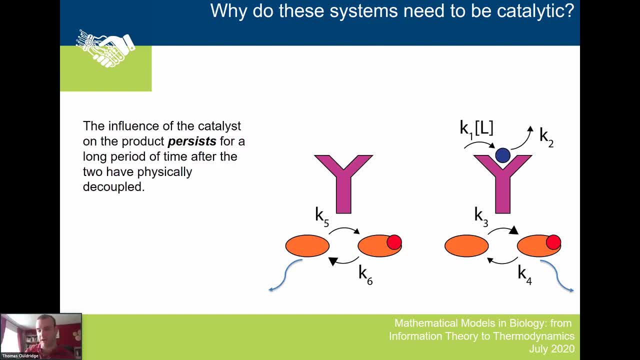 phosphate from ATP and giving it to your downstream readout, But because one of those reactions is miles faster than the other. that's effectively all you see. Similarly, the phosphatase accelerates both- Where's my cursor? Both the giving phosphate back to solution and binding phosphate solution, but because 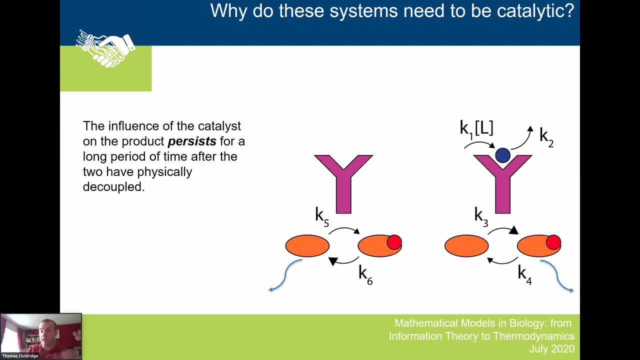 binding phosphate from solution is so much less favorable than giving it back to solution. you only really see the phosphatase dephosphorylates it. So you get these cycles and you get the ability to turn on or turn off, but you only get that because 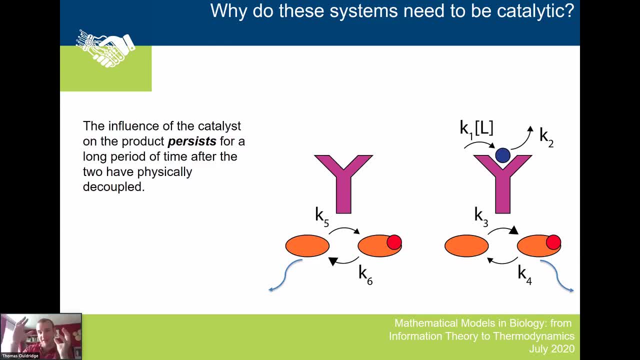 these two processes are actually microscopically different from the other, because you only get the from each other and in going around a circle- uh, back to the start- you've burned one molecule of atp. is that roughly answering the question? he says: got it, yes, brilliant. 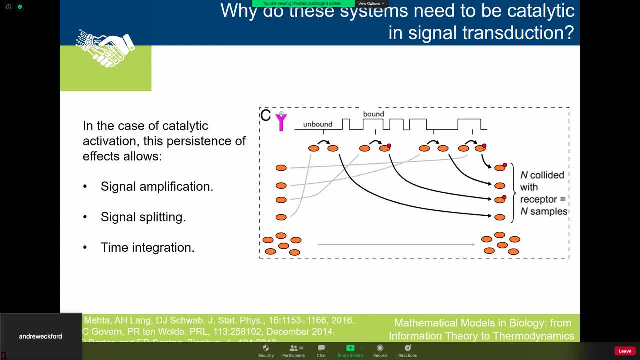 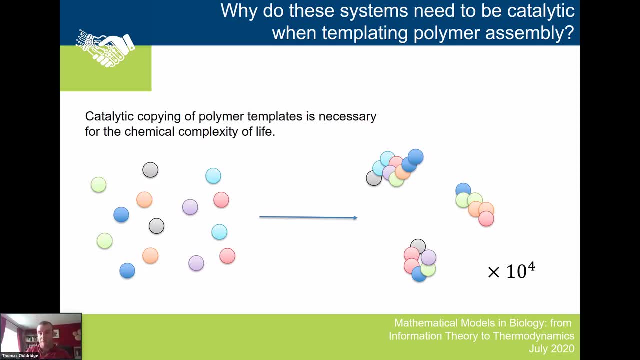 okay, so so that's how it works for a signaling cascade. how does it work? why is it important for templating? so in a human cell there are about 10 to the 4 distinct proteins with completely different structures and completely different sequences of amino acids making up those. 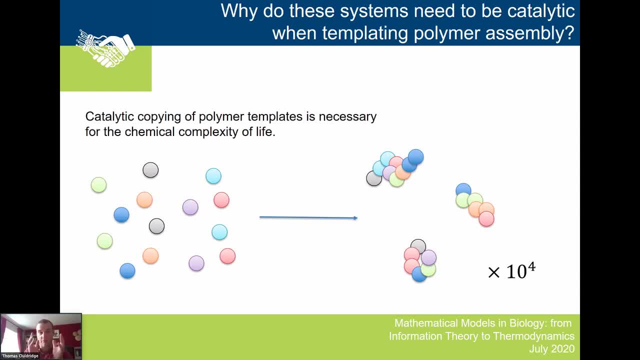 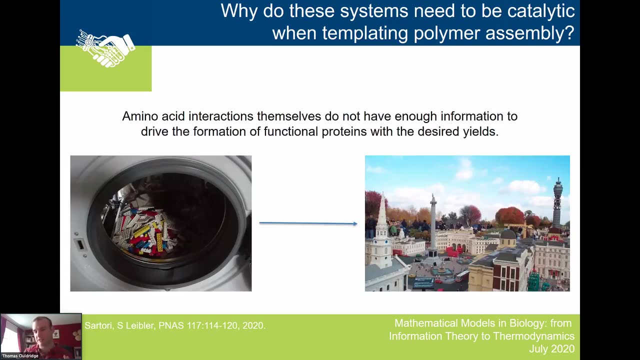 structures. those 10 to the 4 proteins are made from 20 amino acids, 20 distinct types of amino acids that are just effectively floating around free in solution. so if you hoped to mix 20 unique types of components in a pool and then get 10 to the 4 specific things assembling out of 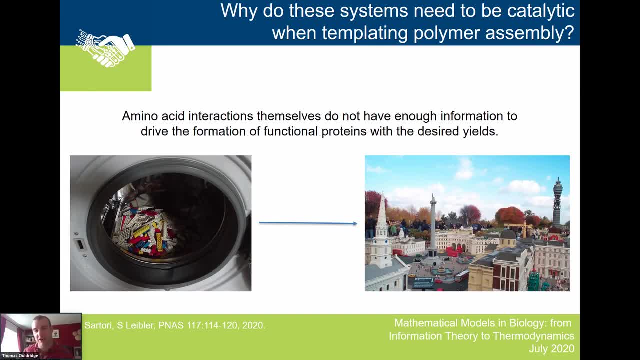 them without anything else, with no other junk. that would be like putting a load of lego bricks in a washing machine and hoping to get a model of london out at the end. you just there just isn't enough information in 20 building blocks to give you precisely 10 to the 4 different assembled. 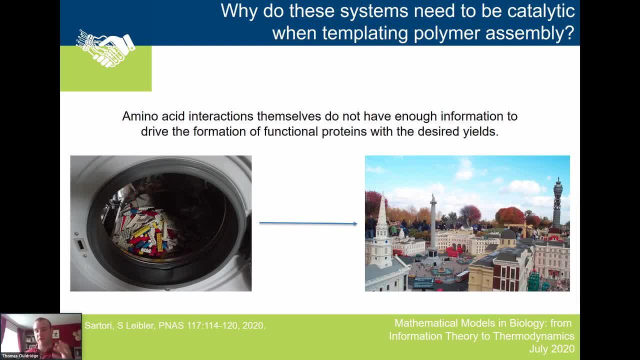 products and indeed that sort of question of how many um distinct products are available from a given set of building blocks um is, is something that's been studied by stanislaus liba and his group. there's a reference down that. so basically you couldn't make proteins just from the amino acids. 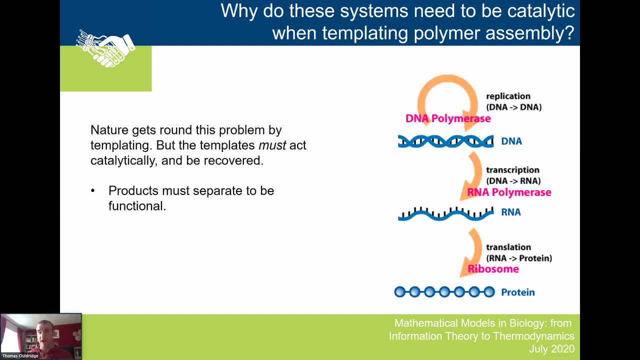 it would be impossible. of course, biology doesn't do that. it uses this central dogma that i talked about before to template the amino acids that are available in the amino acids and then you can. then you can create the sequence of amino acids using uh, rna and eventually the dna sequence. so 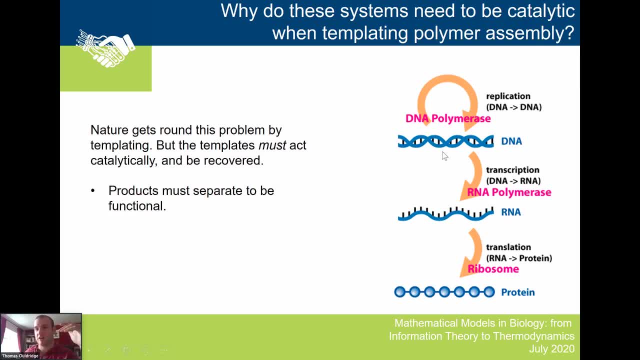 the rna in this context is really just a, an intermediary messenger. there's a sequence in the dna template that is used to direct the assembly of the um, uh, of, of the protein of amino acids, into the right sequence, and when you've done that, there is then enough information. 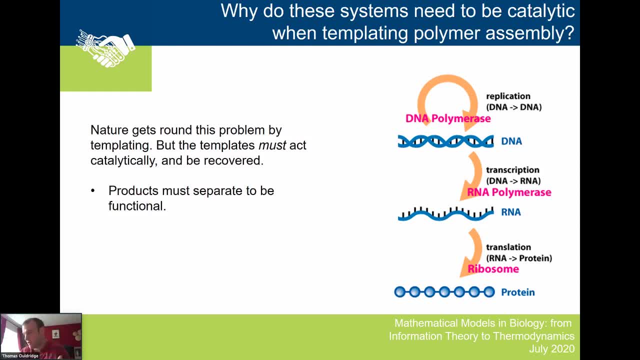 that they can fold into the structure because you've already chosen the reactants, uh, the component and the order in which they appear. so, templating is used to make proteins from dna. this won't be surprising anyone, but somehow i think it's often undersold that these things must act catalytically. um, for a start is no use if your 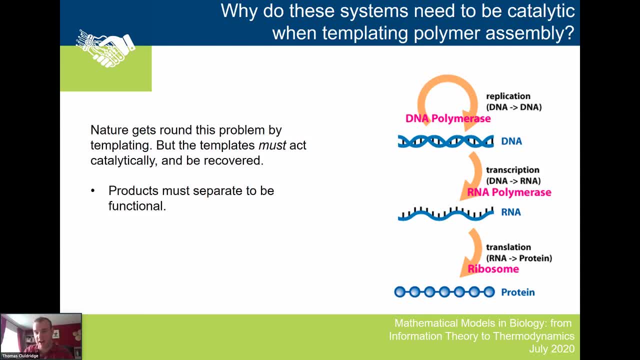 protein stays stuck to your polynucleotide. it needs to detach and go off and have an independent existence and do whatever the protein is supposed to do. but arguably more deeply if you can't reuse the templates having made your protein, if, if and remember. in this case, rna is just really an intermediary messenger and we could, we could. imagine that we were making the protein directly from the dna. if you couldn't reuse the dna sequence to make another copy of the protein, then every time you wanted a new protein you'd have to make a new dna from scratch. and that's actually harder than making the protein, because you've only got four ingredients for your dna and it needs to be. 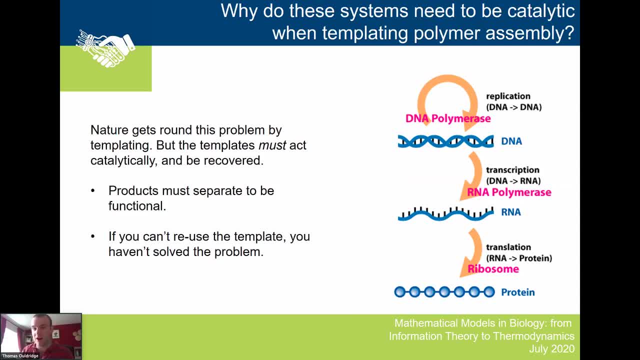 three times as long, so you'd actually made the problem worse if the dna wasn't acting as a catalyst. so, fundamentally, without templates acting as catalysts, you can't um solve the problem of uh biological complexity. so i would argue that this is the most important class of process. 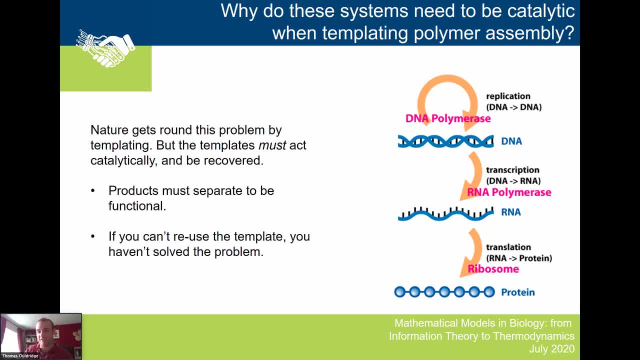 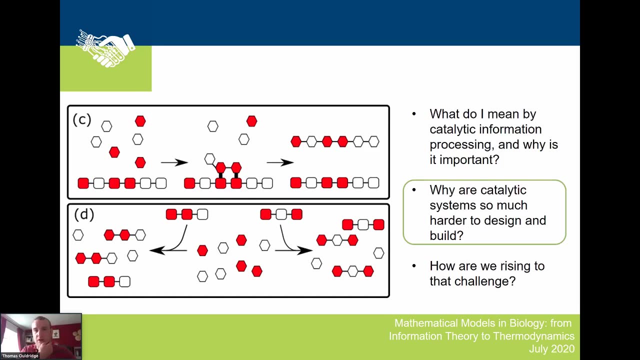 in living systems. um, and i i think to some extent people haven't really thought about it very much from this uh perspective, but when you do, you get some really interesting things coming out okay. so hopefully i've convinced people that, um, some processes in living systems are catalytic. 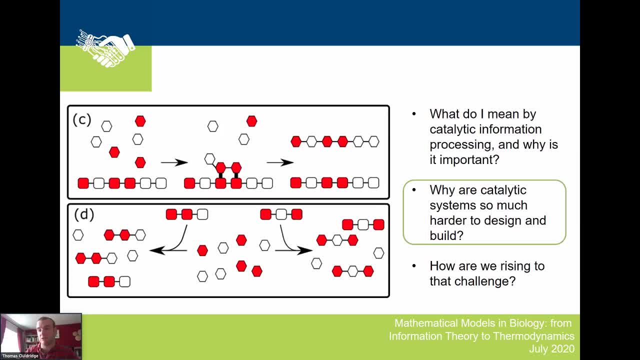 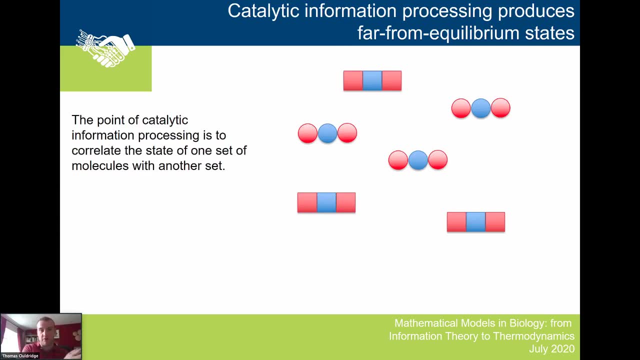 and it's important that they are. so now i'm going to talk about why catalytic systems are really hard to design and build. so the whole point of the processes i described to you before- both the templated uh production of polymers and the um signaling arch architectures- is that what you're trying to do is. 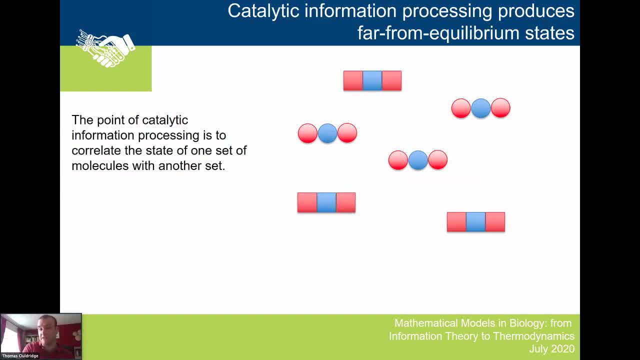 correlate the state of one state of set of molecules with a state of another set of molecules. so, in the case of the signaling, you're trying to correlate the state of the receptor with the all, the state of the readout with that of the receptor. um, in the case of the templated copying, you're 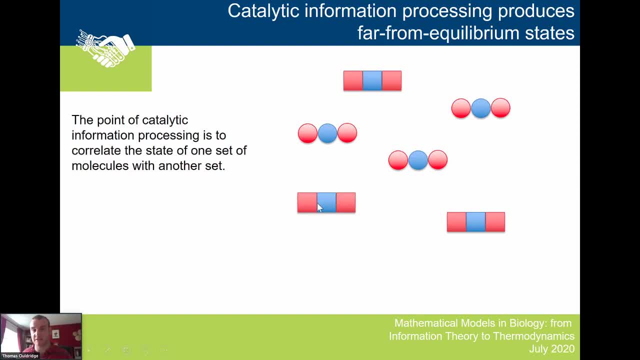 trying to correlate the state of uh templates, which i've represented as three site templates, in this case red, blue, red- with the state of a load of products, daughter polymers, which in this case are also red, blue red. um, and when i say correlate, what i mean is that, uh, in principle i could have red, blue, red and then 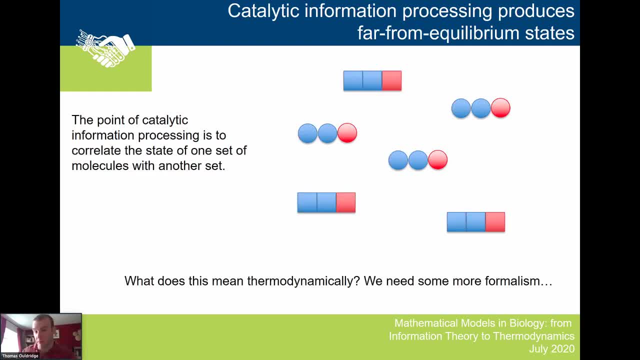 produce loads of other red blue reds, but if instead, my templates are blue blue red, i produce blue blue red. so, um, in principle, the template sequence could be anything, and i need to be able to produce, uh, any, uh daughter polymers as possible. so, um, the sequences, there's a, there's some. 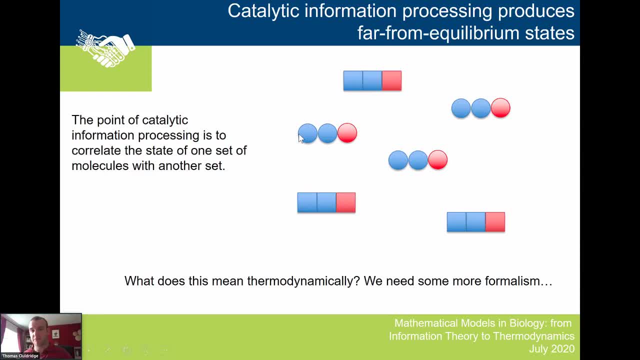 distribution of of these copy uh sequences, but they're strongly correlated with the distribution of templates that are present in the system. so what does this actually mean thermodynamically? well, to do that, we need to go a bit more formal, and i'm going to be leveraging a lot of what udo and massimiliano said over the last two days. 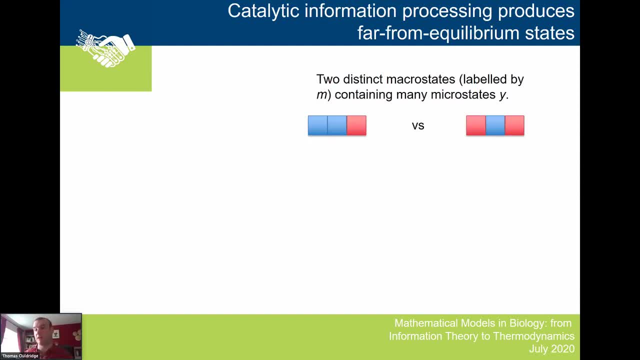 so, as udo described, i'm going to be working at the macrostate level, which i've kind of been doing informally already, which is that i'm kind of going to be describing things like polymers as blue, blue red or red blue red, which might correspond to. 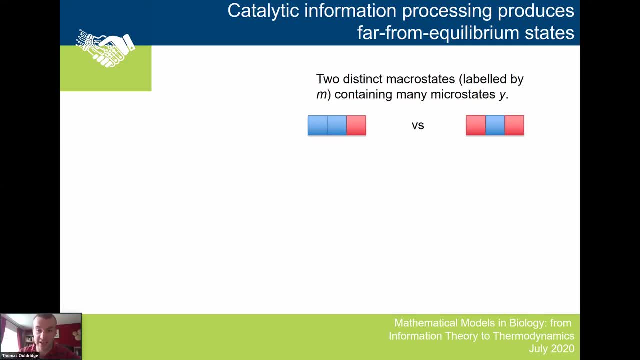 a a t or um t a t as a sequence in a polynuclear type. now, for a given uh set of uh, for a given sequence, there are multiple possible microscopic configurations, which i'd call microstates, uh. but what i'm doing is i'm lumping all of those microstates. 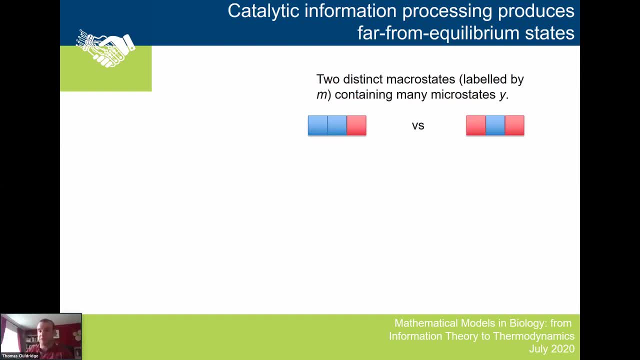 into one macrostate or another. which is this sequence or that sequence? so the in general um, the system uh will be in some distribution of microscopic configurations, py. so it's a probability distribution of microscopic configurations and in general that won't be equal to the equilibrium distribution which is just given by the boltzmann distribution here. 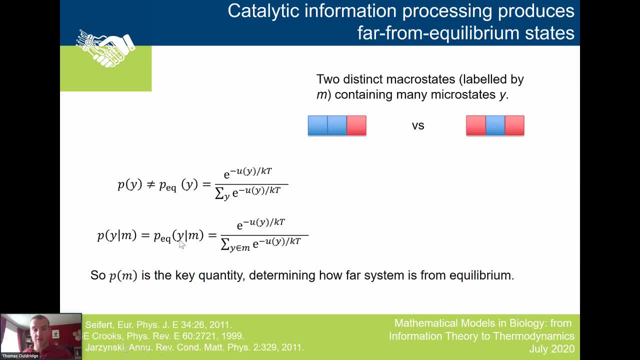 um. however, what i am going to assume- and again, udo covered this in his talk- is that these macrostates are well defined, in the sense that these macrostates are well defined in the sense that there's a separation of time scales, so the system equilibrates effectively within the microstates of 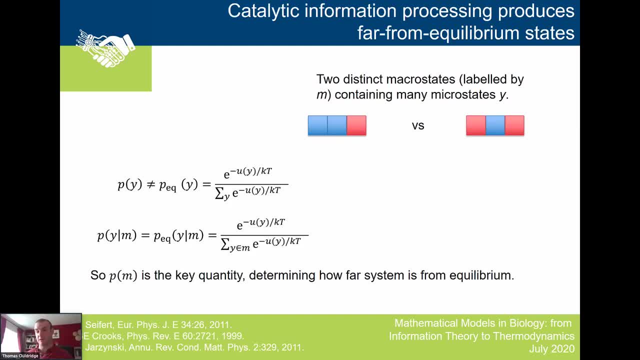 one macrostate but doesn't equilibrate between the macrostates. so, formally speaking, what i'm saying is that, given that i'm in a macrostate m, the y states are distributed according to the boltzmann distribution, but i can't guarantee that two microstates corresponding to different macrostates. 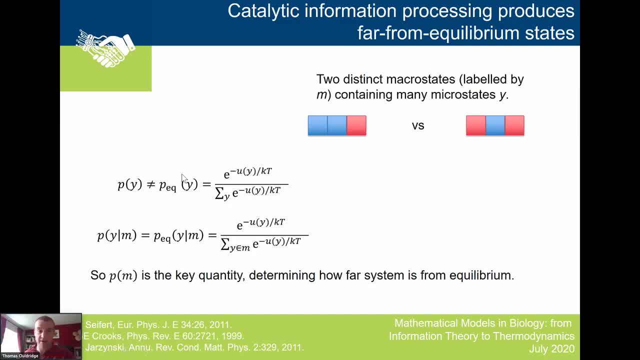 are in equilibrium. what this means is that the macrostates are well defined, in the sense that the, the probability distribution of the macrostates, is the key quantity and that tells me whether i'm in equilibrium and how far away i am okay, so, in general, the distribution over macrostates, i 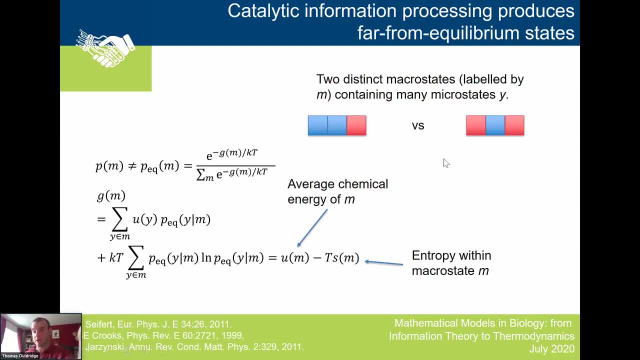 what's the probability i'm in blue, blue red rather than red, blue red or any other sequence? in general, that won't be equal to the equilibrium distribution, and the equilibrium distribution is again just given by a boltzmann factor, but here instead of the energy as a function. 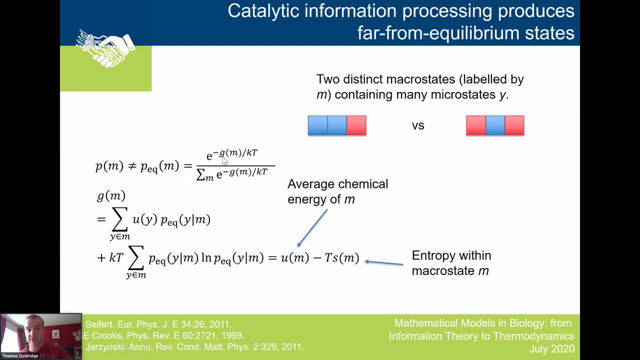 of the coordinate, you've got the macrostate free energy, which is just the combination of the energy within that macrostate, the typical energy within that macrostate. so are the configurations of blue, blue, red? are they low in energy or not? and if they are, g is low and that makes you very. 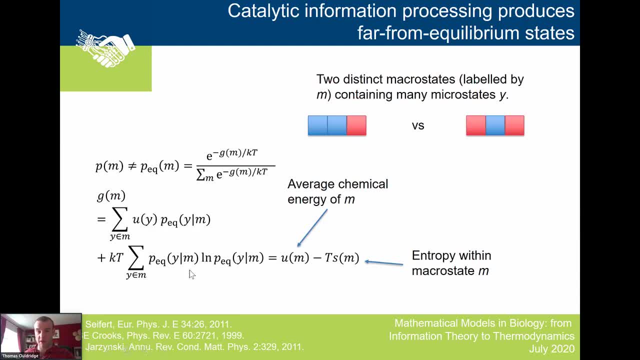 common in equilibrium, but also a contribution from the entropy. so effectively, how many microscopic are there within the macroscopic one? blue, blue, red? if there are a lot of microscopic configurations, that gives a positive contribution, um, to the entropy, um and uh, that makes it positive contribution to the entropy of the macrostate, which makes the free energy lower. and again, 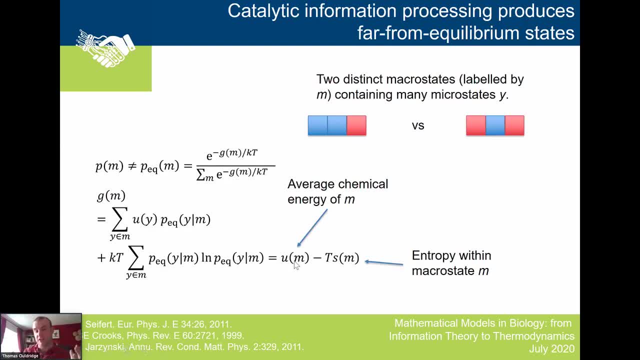 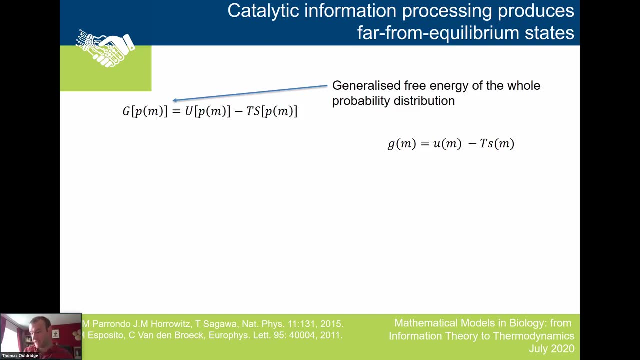 makes it more common in equilibrium. so you've got the, the average energy and the number of states. uh, basically- and i again i don't think this should surprise anybody, um too much. who's familiar with biochemistry? okay. so perhaps a slightly taking a step further is to say: i now want to not just talk about the free energy. 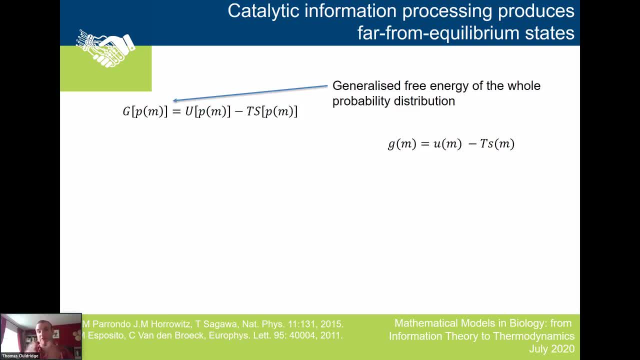 of a given uh macrostate. i want to talk about the free energy of the whole distribution over macrostate. but i want to say what is the average energy of the system, given the probability of being in state blue, blue, red, state red, blue, red, etc. minus uh temperature times the entropy. so how? 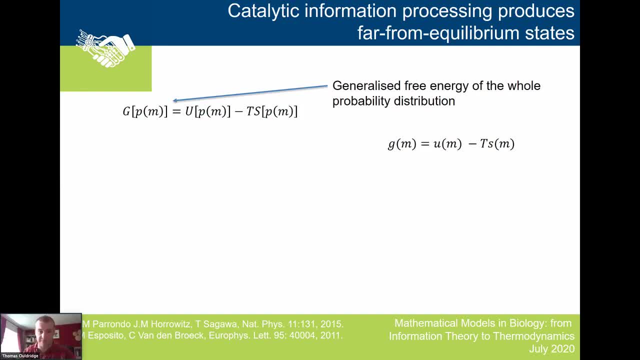 uncertain how many states, uh, am i occupying? now the average energy is just given by taking the probability that i'm in a macroscopic configuration and multiplying by the energy of that macroscopic configuration. nothing special. but the entropy splits into two terms. one of them is the entropy a. 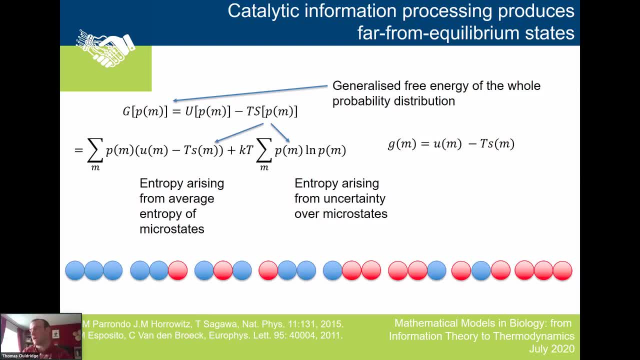 showed on the right side and on the top, left and at the bottom, is a configuration of the energy itself. so it's used for prospecting, so something above the average level, something higher in lightness. so what that actually does is it helps us perform a bigger schizophrenia. 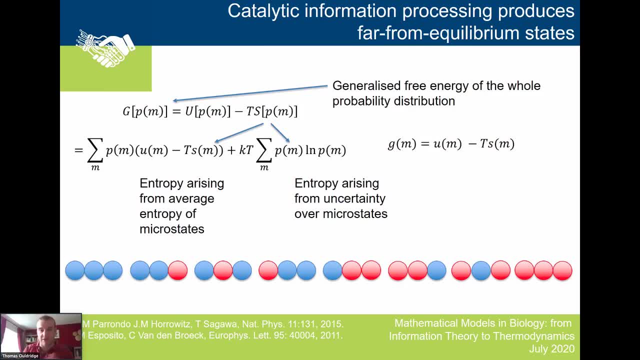 why, demonstrating a nearly signal in this situation? i'm out of my head. what may he be doing now? i'm without it, and so, for example, thin air, or didn't it leak the same amount of energy out of the sun? i'm cutting one of the anatomical 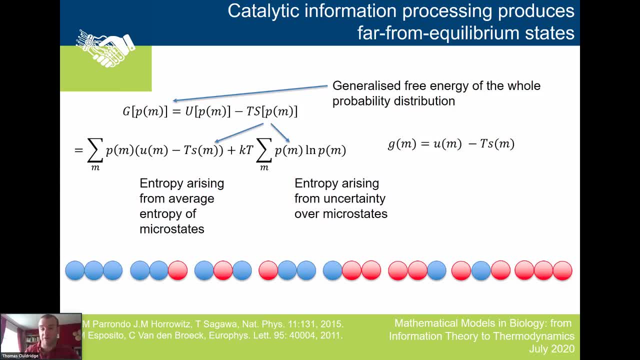 Hallway system and it's actually using a voltage waveform, so the heat output from air and into your system comes from your system as well. so that's exactly what this will do. if you wonder why didn't we do this? this first term is the term that corresponds to how much microscopic wiggle do I have given that? 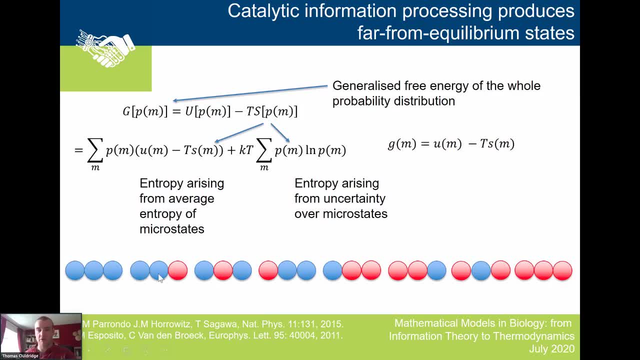 I'm in blue blue red, And the second term corresponds to how certain am I that I'm in blue blue red rather than blue red, blue red, blue blue, et cetera. So this second one, 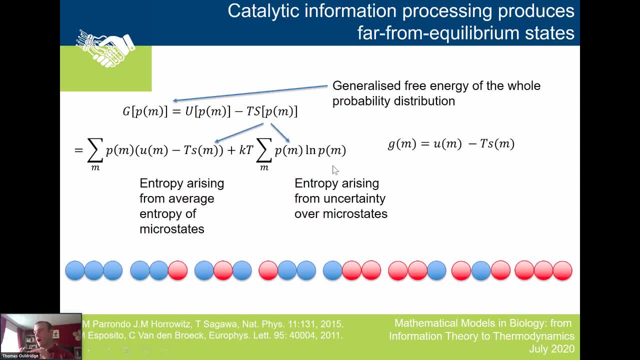 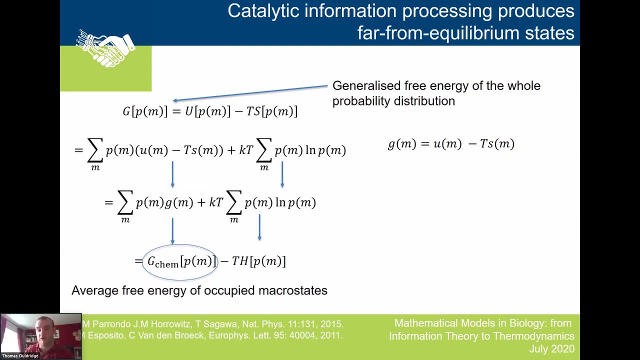 is really the informational thing that we're interested in. It tells us how much information is there in the sequences that are present in the system So we can rewrite this as what I typically call a chemical-free energy. so how much chemical-free energy is there in the system? 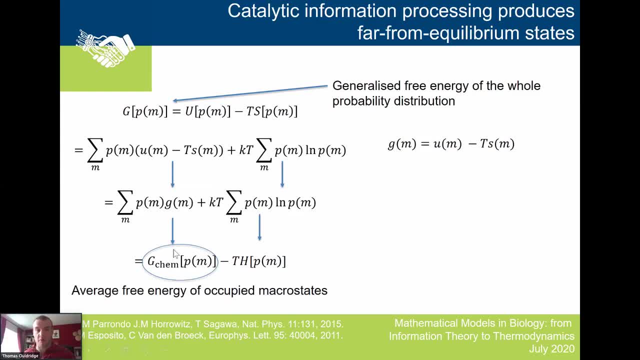 And this is what you'd be very used to from biology, in terms of talking about the chemical-free energy of a bond, Chemical-free energy of a bond favored by low energies, disfavored by the fact that there's no energy in the system. So this is a good example of a bond. So we'll talk a little. 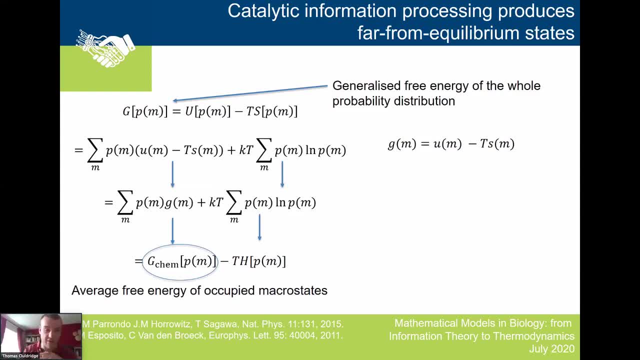 bit more about that. But before I move to the next slide, I'm going to talk a little bit more about microscopic configurations are restricted because the things are stuck together. right? this is just the normal chemical free energy. the second term: this is the entropy. due to the uncertainty over 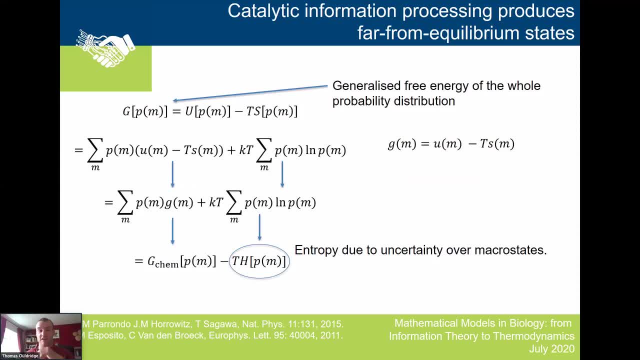 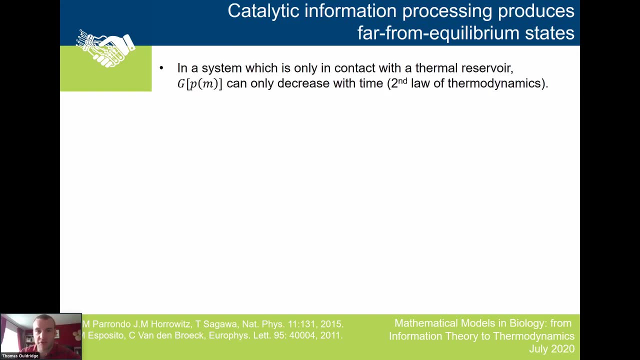 macrostates. and this is basically. it's small when you're very certain about the macroscopic configuration you're in, and it's large if you're very uncertain. so why is this generalized free energy useful? well, it turns out that- and again this was touched on by Massimiliano- is that? 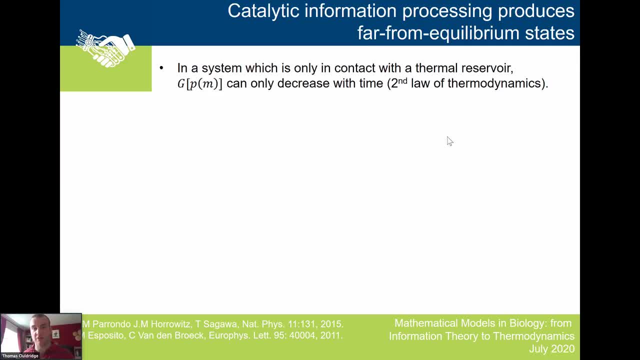 if you're only in contact with a thermal reservoir, ie if you're not being pumped, if you're not being continuously supplied with fuel, your free energy, your generalized free energy, can only decrease with time. this is the second law of thermodynamics. in this context, 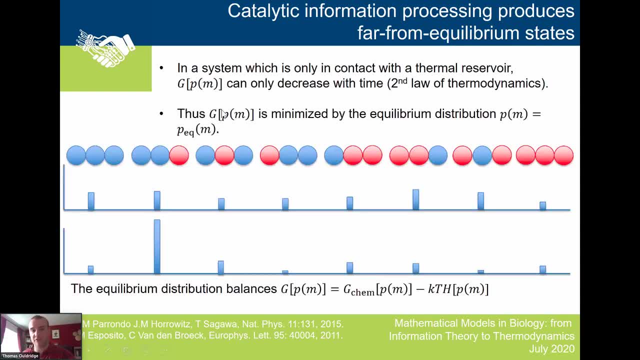 so what that means is that generalized free energy is minimized by the equilibrium energy and the equilibrium energy is minimized by the equilibrium energy distribution over macrostates, So that equilibration distribution could be fairly flat. So if all of the chemical free energies of all of these different macroscopic configurations 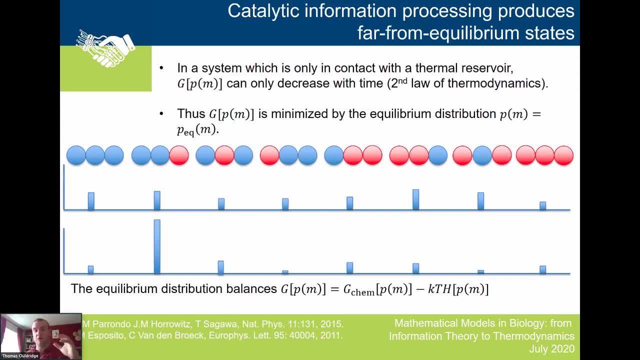 are roughly similar, then the system will say: OK, all of these are pretty much equally favorable and will spread as much probability as possible over the different states. You'll end up with a fairly flat probability distribution. However, if one of them say this one: 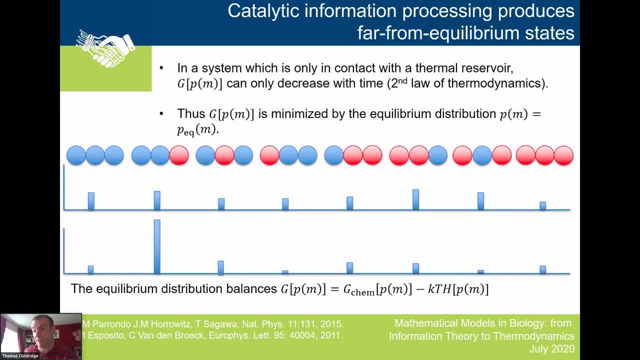 has a much lower chemical free energy than all the others, the system will tend to occupy that configuration. So basically you can pay for a low entropy with a low chemical free energy And again, hopefully that doesn't surprise people too much. The slight difference here is that we're 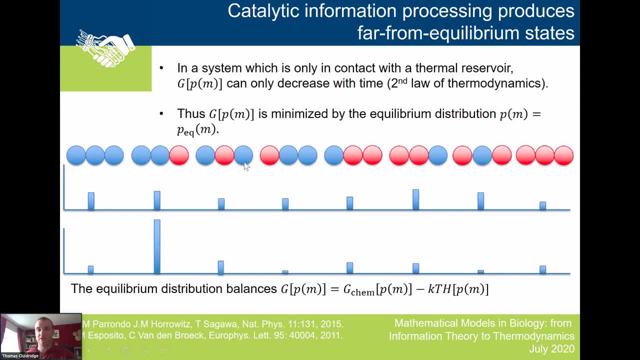 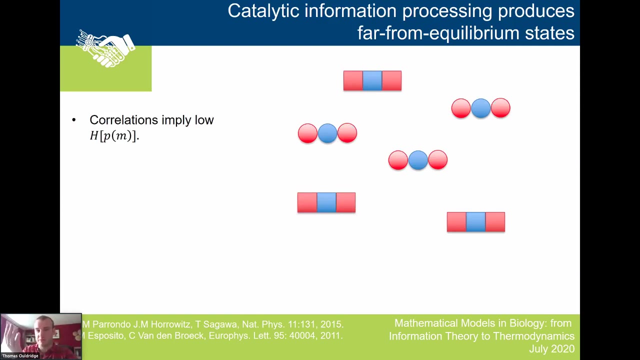 talking about this sort of informational entropy, which is related to which macroscopic configuration you're in, and the actual microscopic entropy associated with the individual degrees of freedom has been all swallowed up into this chemical energy. All right, So in catalytic copying we create correlations. 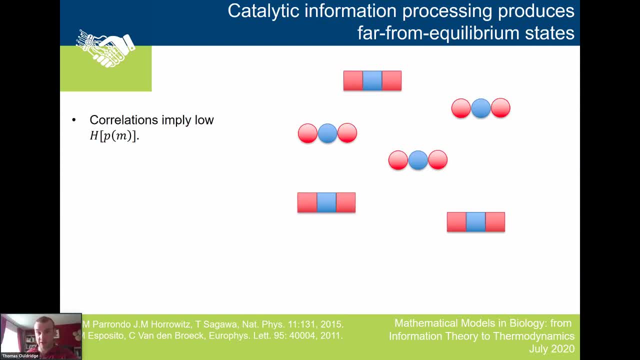 between inputs and outputs. So this means that the entropy, which is low, there's low uncertainty in the state, because we can have states that look like this or we can have states that look like that, but we can't have states or we tend not to have states. 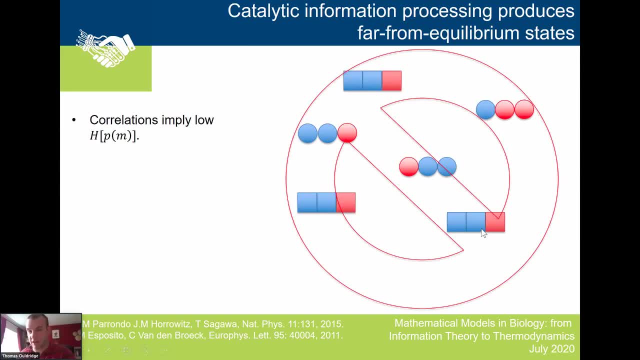 where the product sequences aren't tightly related to the template sequences. so we've got a low entropy. however, there's no direct physical interaction between the templates and the copies. as i said before, they're catalytic. at the end of the process the copy have got to detach. 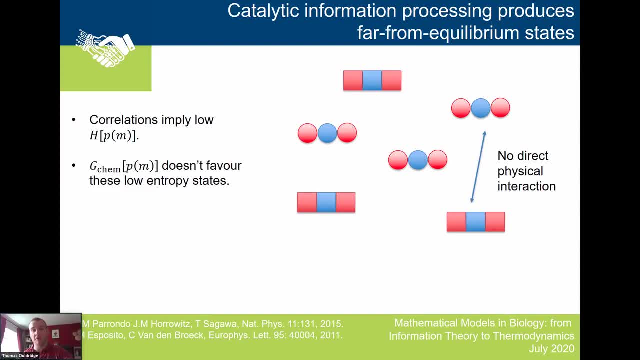 they've got to go off and have their own existence. that's not only what actually happens in the cell, but it's actually fundamental to to to how these processes need to work. okay, so there can't be a direct physical interaction? and if there is no direct physical 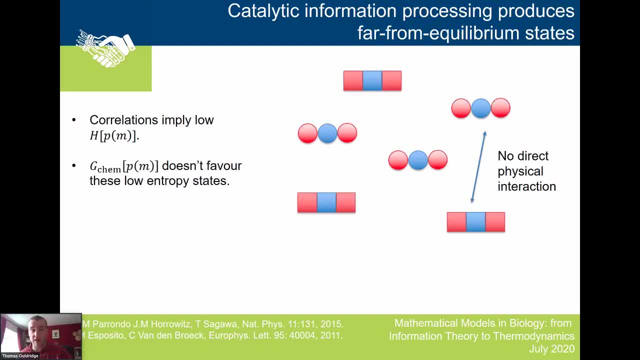 interaction. what that means is that the chemical free energy can't be more favorable in this state than in that state systematically, because there is no interaction between this template and this product And therefore there's no reason why the correct sequence that you want needs to. 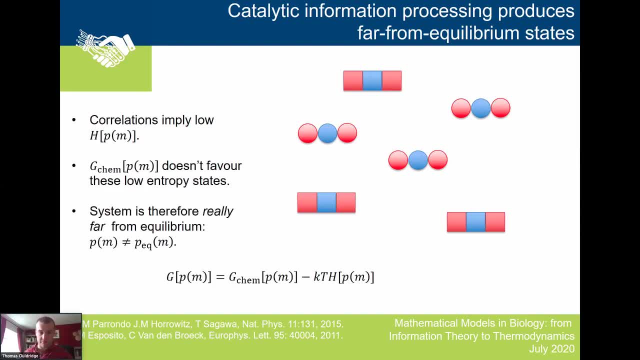 be favored in equilibrium. So the conclusion- and this is really the one thing to remember from my talk- is that these catalytic information processing systems, they produce states that are really far from equilibrium, And when I say really far from equilibrium, I mean at the 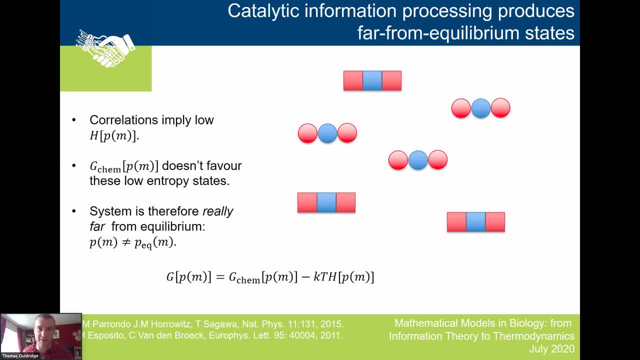 macrostate level about as far from equilibrium as you could possibly imagine. The RNA, the production of an RNA sequence from its DNA. let's say it's I don't know a hundred bases long, which is a short piece of RNA. Typically speaking, that sequence will be: 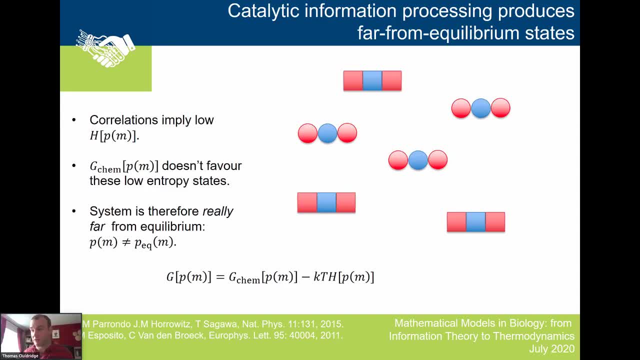 produced in a cell with pretty high accuracy, order. a hundred percent of the sequences are correct, And so they've managed to pick one sequence from four to the power of a hundred, And there's no reason why that one sequence is actually any more energetically. 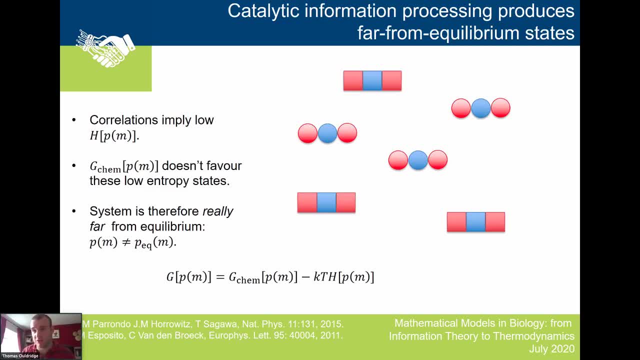 favorable than any of the others from that distribution. So that is stunningly far from equilibrium And my argument is that you really can't think about the properties of these processes without taking that into account, And I would make the case that in the past people have tended to study these systems and ignore that fact. 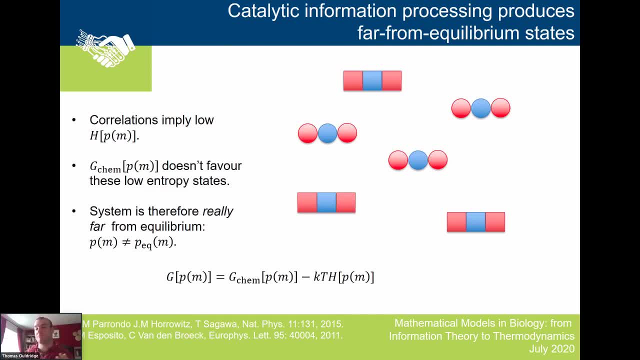 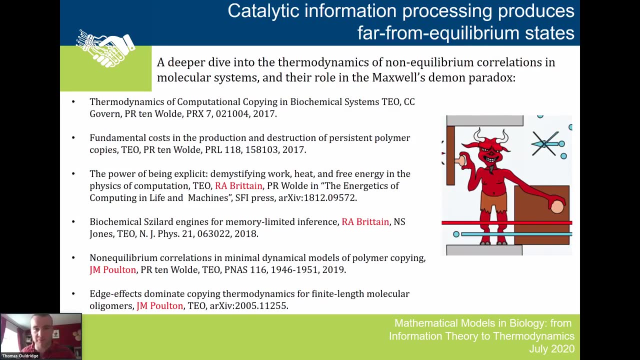 And that's why I'd argue, we're in a position where we can't actually build catalytic information processing systems, as we'll explore in a second Okay, So ordinarily I would now dive very, very deeply into the thermodynamics of non-equilibrium correlations in molecular systems and also. 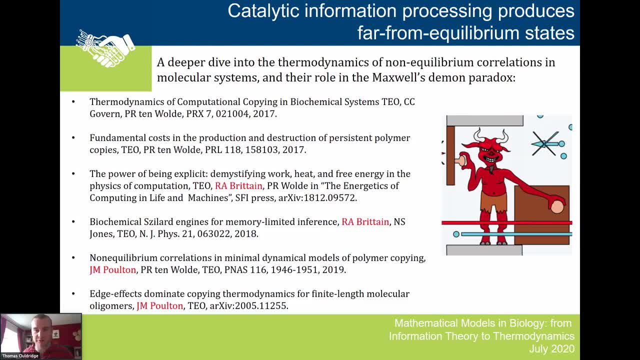 get into a load of fights about the interpretation of Maxwell's demon and Szilard's engine. But today I want to focus a bit more on the sort of like the practicalities of what I've just said, rather than the fundamental physics. But here are a load of references which I'm 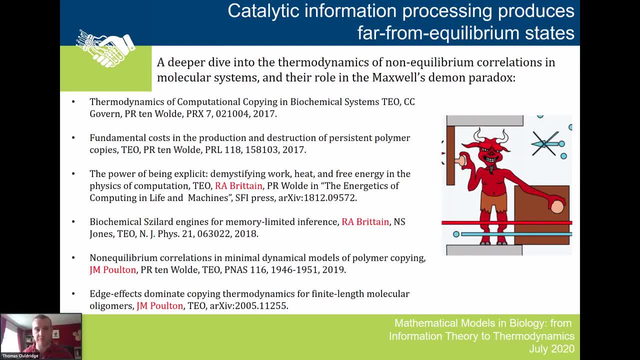 I've shared the slide, So hopefully everyone can see them if they need to. I'd like to highlight Rory, who I think is in the back right hand corner. He's a good person too. He was a good friend of mine. He was a good friend of mine. He was a good friend of mine. 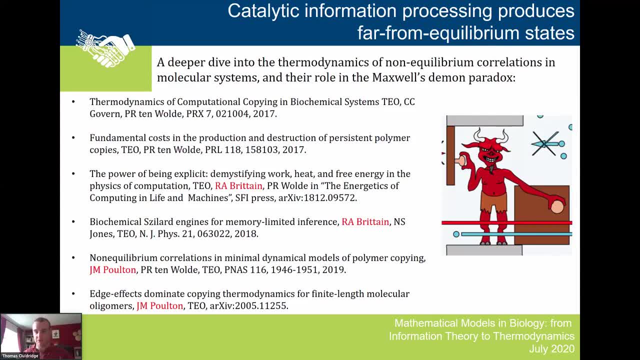 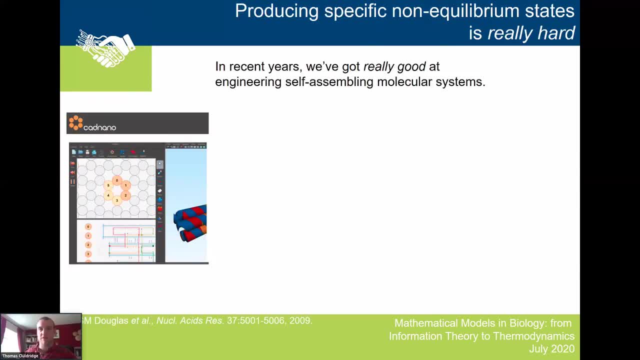 who I think is in the audience today, and Jenny, two of my students who did a lot of this work. Okay, so, in recent years we've got really good at engineering self-assembling molecular systems And my background is in DNA nanotechnology And in DNA nanotechnology. what you can do is you say: 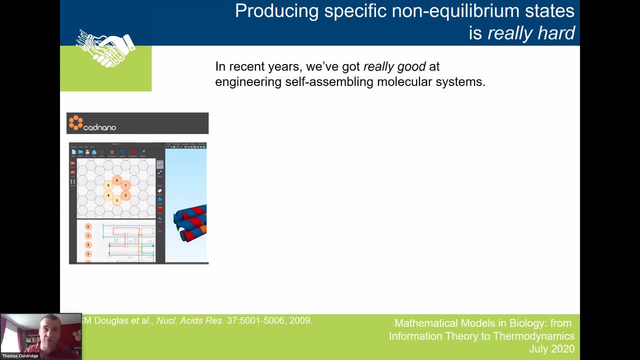 I want to build a structure of a given shape. You sit down either with a pen and paper or a CAD tool like CADnano. you draw your shape. you work out a load of sequences of DNA strands that are complementary in such a way that they'll tend to form that shape in equilibrium. 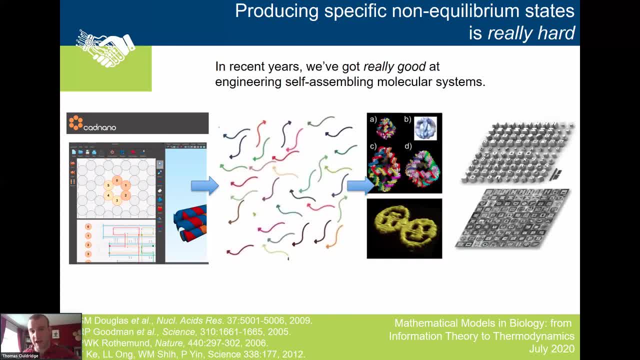 You mix them up in a pot and you cool it down and the shape comes out at the end for you exactly as you want it, And people have been able to assemble remarkably complicated things in this way. I don't know how. hopefully, these 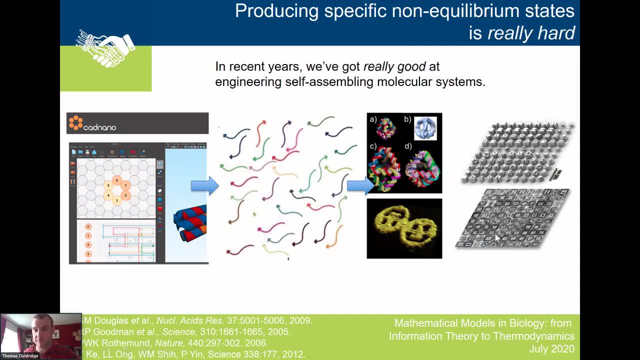 structures here. these are real electron microscopy images of assembled structures. these aren't pictures, So they're able to assemble. this is a picture. this is the assembled structure, So self-assembly really impressive, particularly with DNA, because we can specify. we know so well that A will stick to T and G will stick to C. we can specify the. 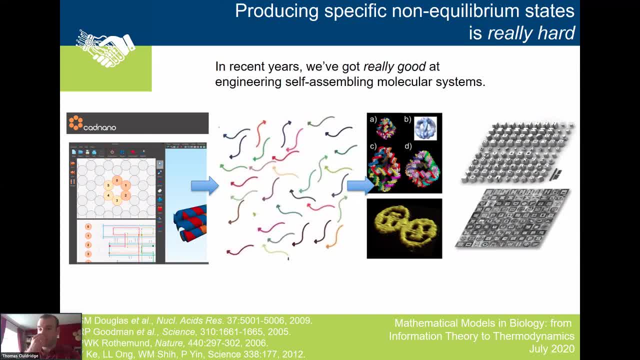 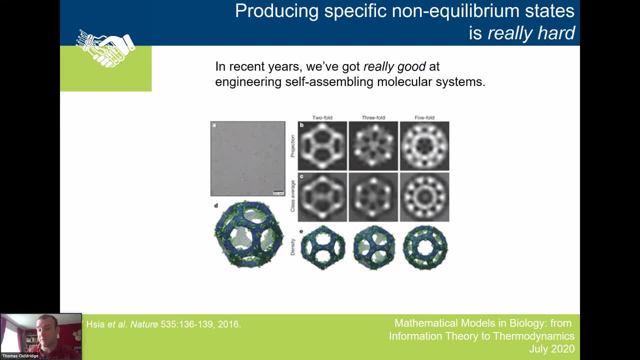 assembled structure with such precision Harder with proteins. but David Baker's group in recent years have been making progress in that direction and have assembled some pretty complex structures through rationally designed protein self-assembly. And it should be noted that, although typically to get the best yield, 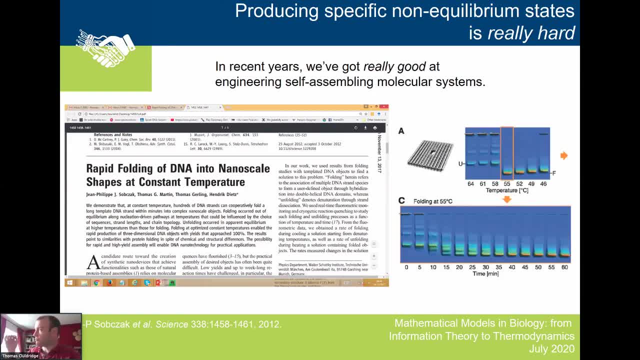 people tend to do a temperature ramp so that you go through the exact assembly point at the right time. If you're careful enough, you can also assemble complex structures At constant temperature, So you really can put a load of ingredients in a pot and watch them. 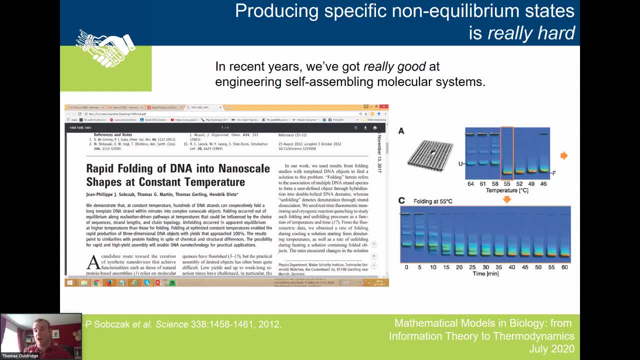 assemble into one of these complex structures, And these structures arguably resemble the complexity and size of the things that cells can assemble in equilibrium as well, So sort of virus, capsids and things like that. We can basically make things that are as complicated, if not more. 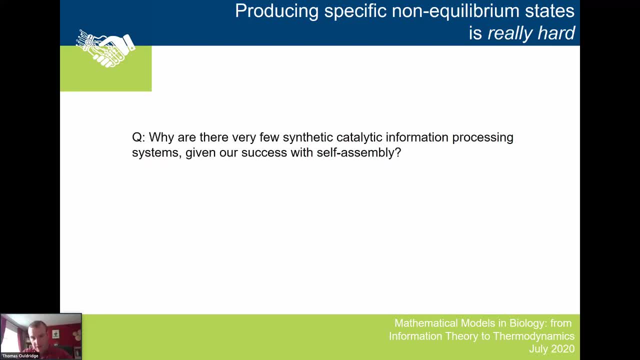 complicated, So we're really good at self-assembly. But there are very few synthetic catalytic information processing systems coming out of the same research And I would you might ask why, especially if you believe my argument of the first half of this talk that actually catalytic information processing is the really fundamental thing, that 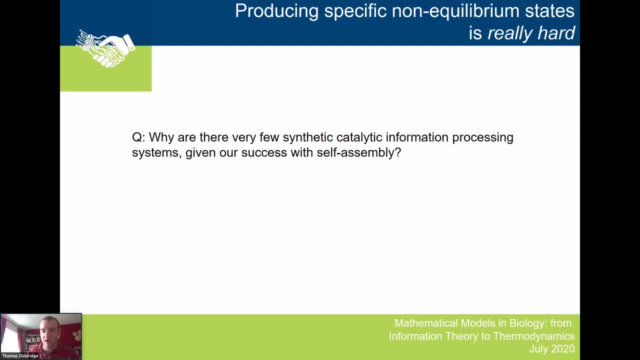 biology that enables it to be interesting. And my answer is: they're hard to engineer because you need strong, selectively attractive interactions For the things to act as catalysts and act as catalysts for the right sequence. So you want to. 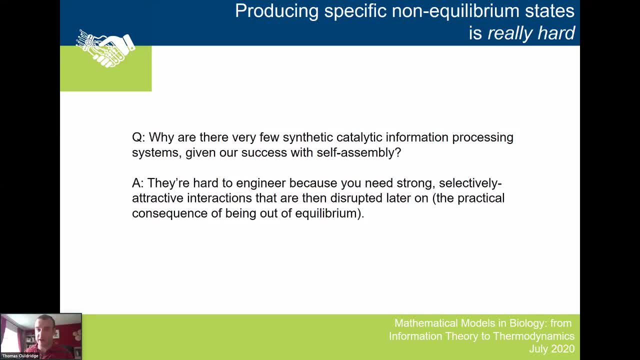 you want to template the assembly at the right RNA, not the wrong RNA. But then the strong, selectively attractive interactions. you need to disrupt them later on. And that's the, that's the practical statement that the eventual product needs to be out of equilibrium. And that is just. 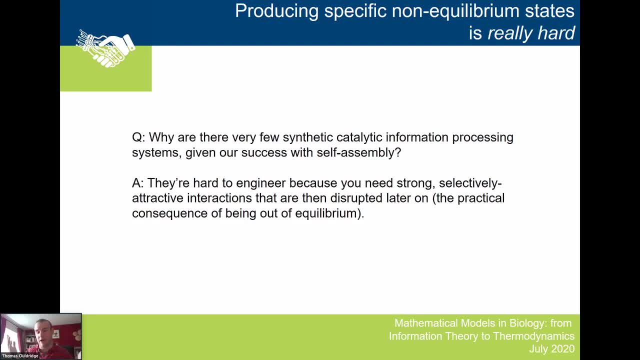 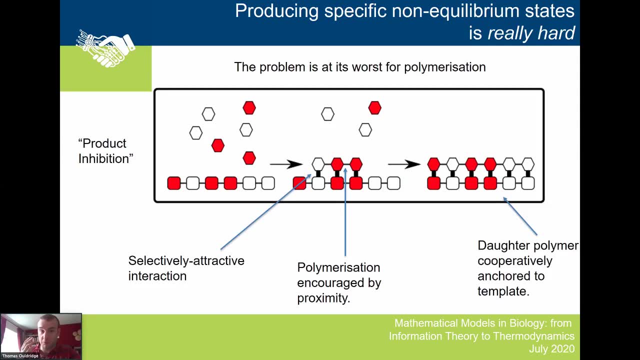 makes it so much harder than being able to mix things together and let them fall to an equilibrium. So- and this problem is worst- for polymerization. So if you want to make one of these polymer copies, like in RNA or DNA, templating, So what happens? let's say, and you could do this very easy, easily. 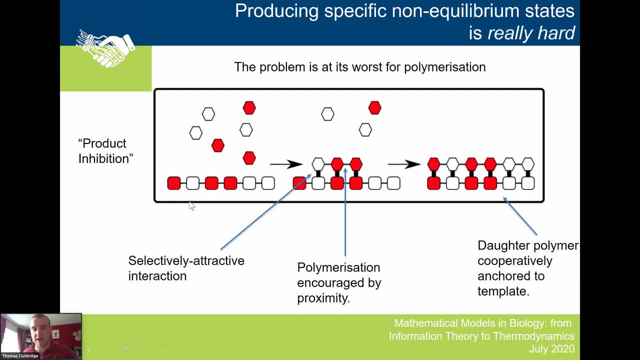 with DNA nanotechnology you could create a monomer template that is complementary to some other monomers in solution and they stick to the template. And because they're stuck to the template, they're close to their neighbors, they bind to their neighbors, they polymerize. 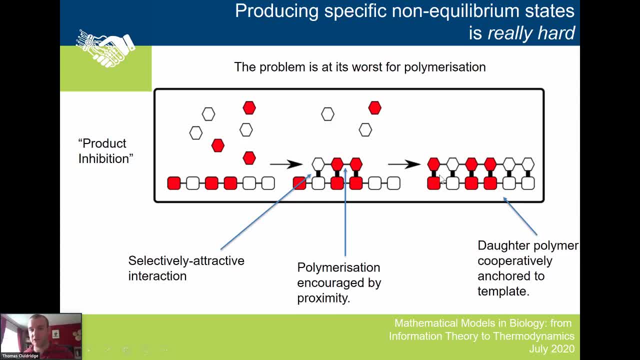 and they form a ladder here where the daughter has the same sequence as the template. This loads of people have done this. this is quite easy. It's effectively self assembly. But at this point the daughter, polymer, is cooperatively stuck to the template. 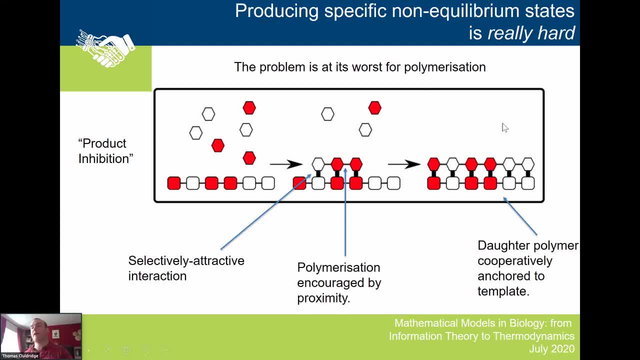 There are six bonds here And you only gain one entropic degree of freedom when you detach from the template. And you only gain one entropic degree of freedom when you detach from the template. So it really is stuck very strongly And this tendency of the copies to stick to the template. 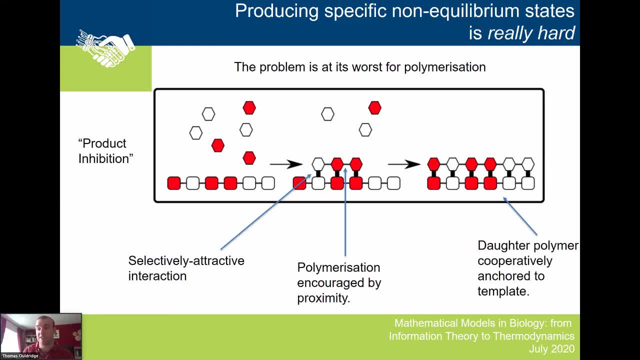 is called product inhibition in the trade And basically people haven't really come up with chemical ways to get around the problem. They instead they'll use things like heat cycling to break these, break these interactions. Okay, it's now 45 minutes. Do I have 10 minutes more? I mean, 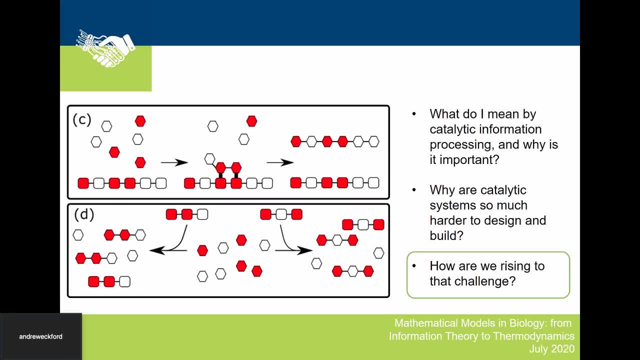 we've kind of stopped for a couple of questions. So I'm going to stop for a couple of questions. Is that okay? That's fine with me. We have a. we're scheduled to have a half an hour open discussion, But I mean we can certainly continue into that, So please go ahead. 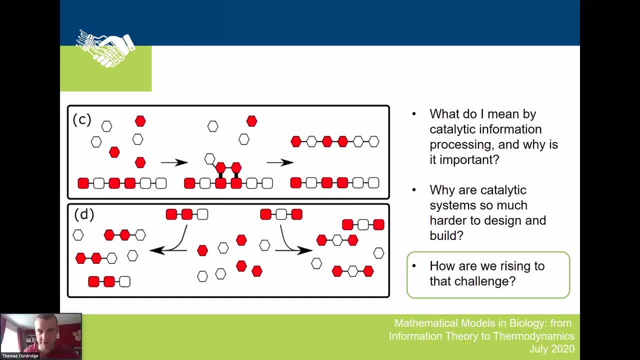 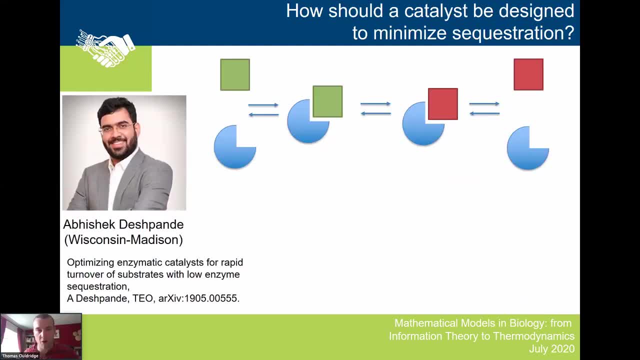 Yeah, okay, great, And please do continue to ask. So. so first of all, I want to briefly mention some work by a former PhD student, Abhishek Deshpande, who's now in Wisconsin, who who asked a very simple question about: okay, if I want to build a catalyst, how do I design? 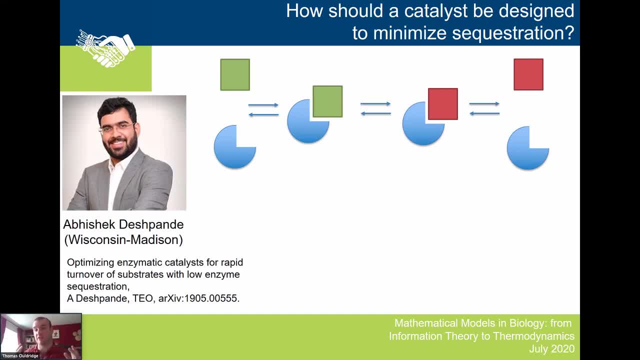 a catalyst so that this product inhibition effectively is minimized. And his is, you know, a very simple model of a catalyst. You've got the catalyst and the substrate they bind, the substrate gets converted into the product and then it gets released, And all of these steps. 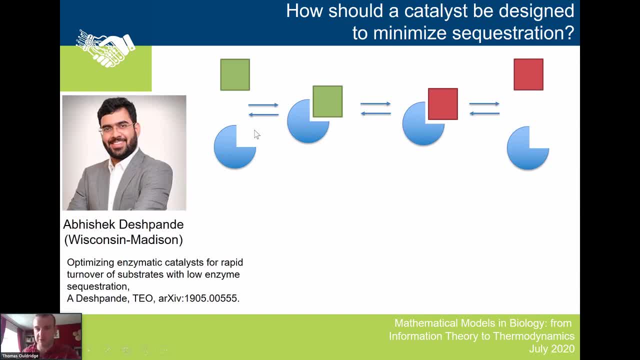 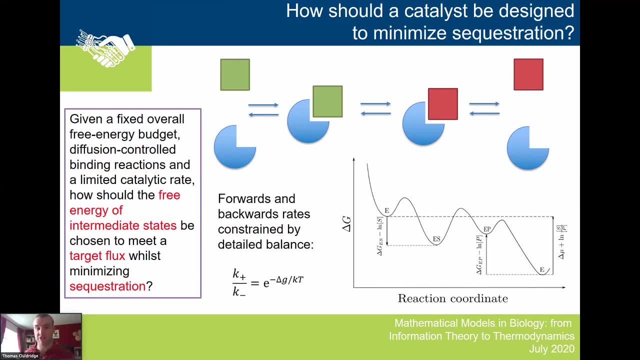 in principle are reversible because we need to. we want to be able to do the thermodynamics. Okay. so he said the question is: given an overall free energy budget, ie an overall change in free energy from going from this state to that state, and reactions that 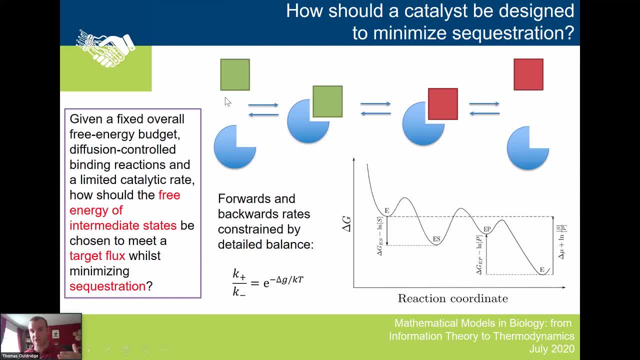 are diffusion controlled, so the binding, these two binding reactions, they're diffusion controlled, so they have a fixed rate rate constant anyway. How can I design my catalyst in the sense of changing the energies of the intermediate substrate and product bound states? 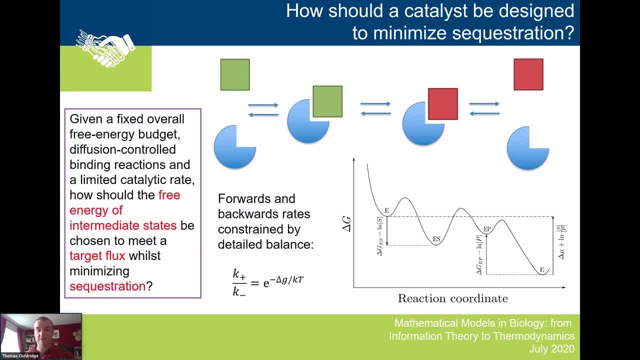 How can I change them to be optimal so that the catalyst has a high flux, ie converts as many substrates into products as possible, whilst minimizing the amount of time that i spend in these intermediate sequestered states? so how do i get as catalytic as possible in some sense? um, okay, and we apply thermodynamic. 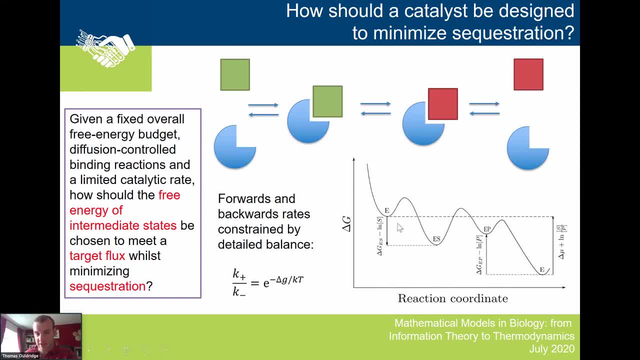 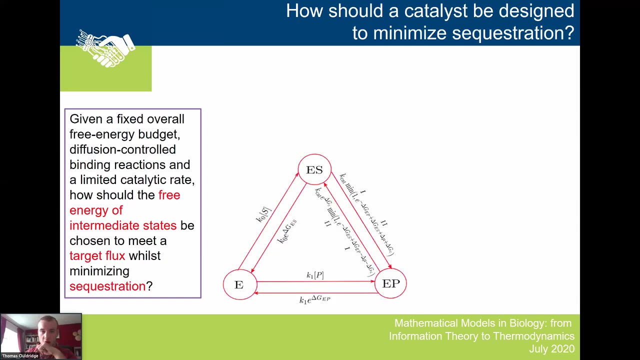 constraints. so the overall free energy change is set and we talk about moving these intermediate states up and down the substrate bound and the product round, and we apply the rule that the forwards and the backwards transitions are related by the, which again was introduced in the first uh talks we saw this week. so, um, this system, um, if you've got isolated enzymes, 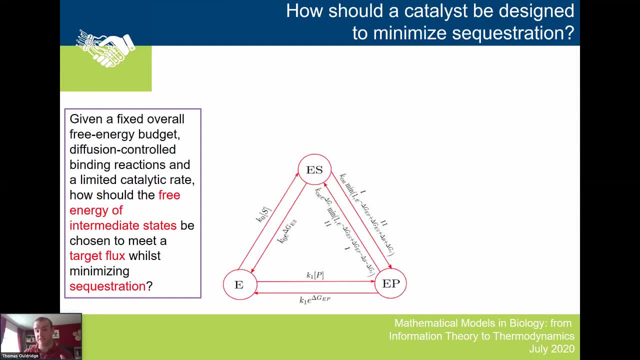 you can. you can analyze each enzyme as a three-state system, which can either be substrate bound, product bound or free. and the transitions? uh, here's a diffusion, limited binding of the substrate and release of the substrate, and that's related by the, the chemical free energy of the of the bond. the only subtlety we have is that the conversion between the product. 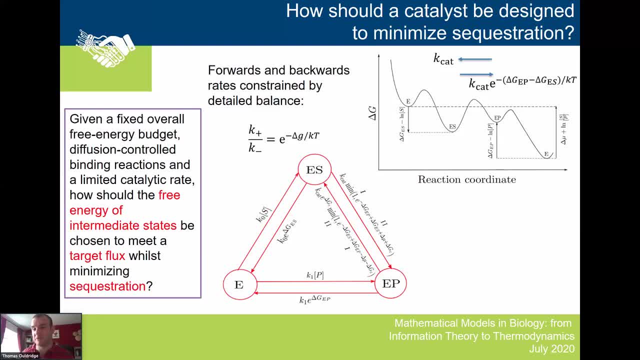 and the substrate, um. you need to make some statement about some maximal rate there. if you allow one of these reactions- the substrate to product conversion- to be infinitely fast, then you get pathological answers which just says: make your enzyme infinitely fast, um. but if you say that there's some fundamental limits, either the forwards reaction or the backwards reaction- 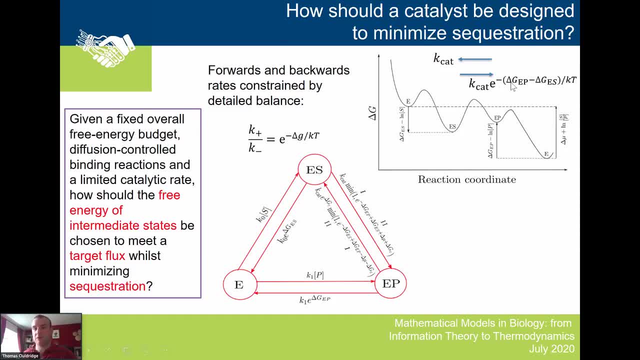 goes at that speed limit and the other one is slowed down. uh, according to this um, delta g uh rule. uh, then you can. then you can make sensible. uh, you can ask sensible questions, um, and then you can. then you can make sensible. uh, you can ask sensible questions, um, and then. 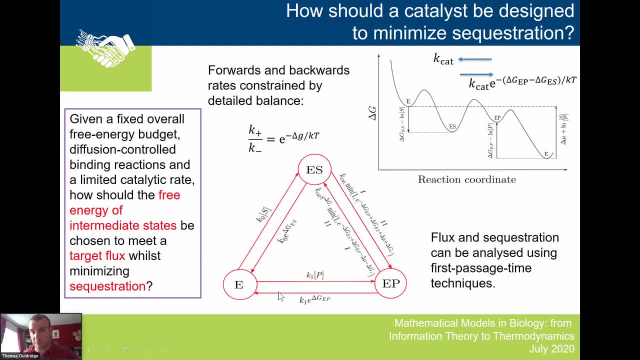 so what you can do is you can, you can solve this system. it's pretty simple and you can analyze the flux, ie the net tendency, the net current for the system to go, to go around a cycle like this: ees, ep, back to e, um and the sequestration in terms of first passage. 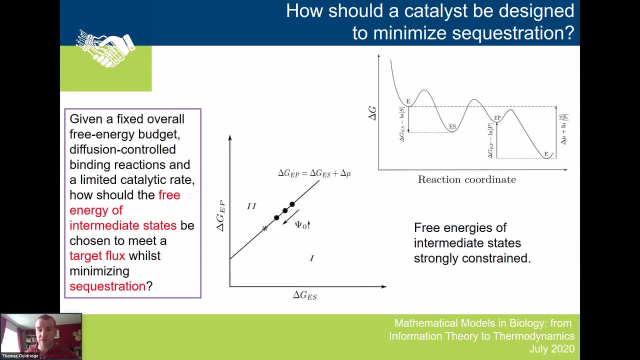 times, uh, of processes, and what you can in fact show is that, if you do this and you want to minimize, um uh, sequestration- ie the amount of time you spend in either this state or this state, rather than free, if you want to minimize sequestration, what you end up doing. so i'm just going to 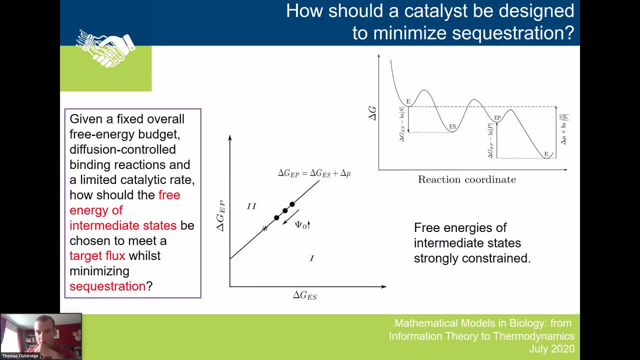 take a drink. what you end up doing is moving towards this line of solutions, uh, which are a fixed offset between the energy of the product bound straight state and the energy of the substrate bound, ie hooked up in a free state of flux. that beni does. there's a difference right there between 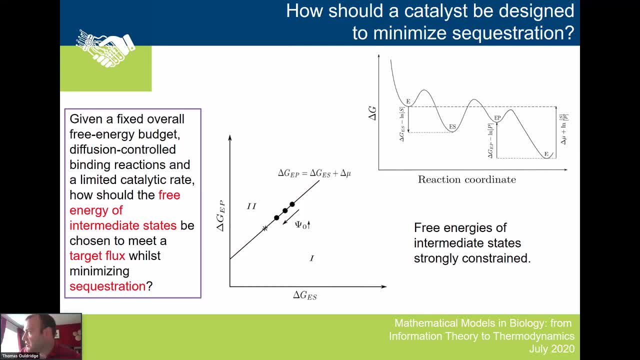 three frequencies. so you know centricино associated with that, which is some intrinsic free energy change, delta, mu plus a log of concentration ratio substrate to products. So really, yeah, this would be like n substrates and m products and this would be n minus 1 substrates and m plus 1 products, And this 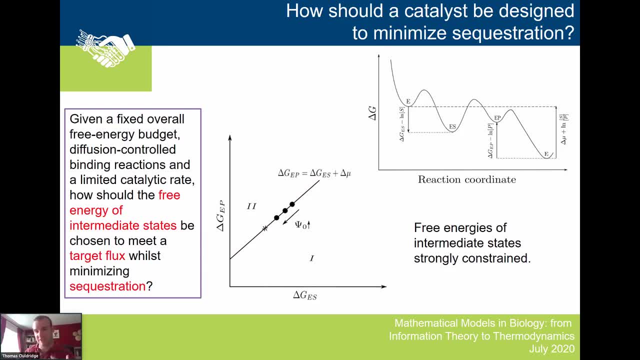 implicitly having something pushing you around a cycle is kind of exactly what we had with the ATP at the start. Is that okay? Sounds good to me. Yep. The questioner says good, Good, Okay. So what happens is that? you're Sorry, just to quickly interrupt again Another. 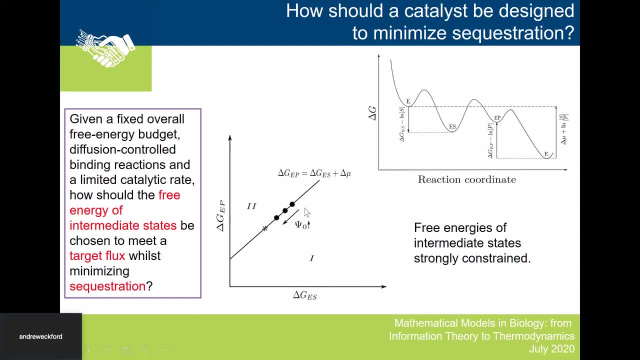 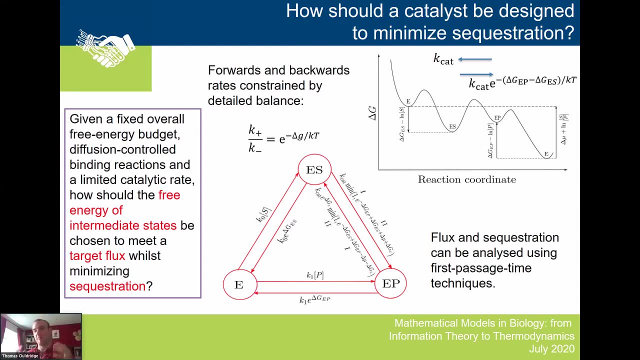 question just popped up. This is more of a statement, which is: the figure should start with E plus S and end at E plus P. Yes, So we, from the perspective of our system, we are. we're treating it a bit like Massimiliano. 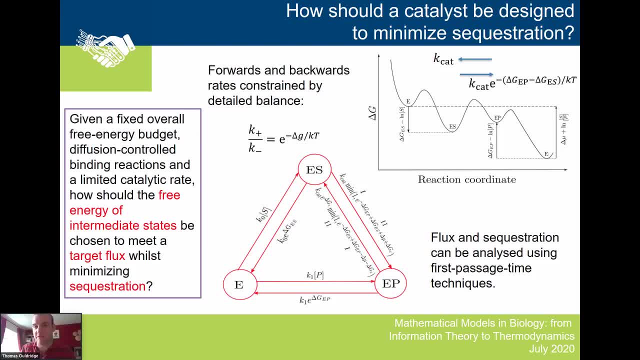 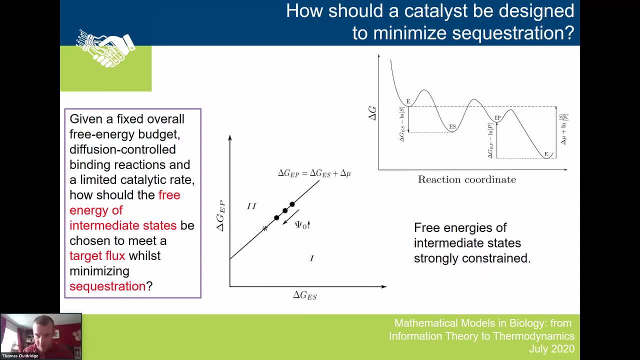 was with with just saying what's the state of the enzyme. And the state of the enzyme is: is E in that configuration? But yeah, I mean, there are, there are different, there are different formalisms that you could you could use, Agreed. 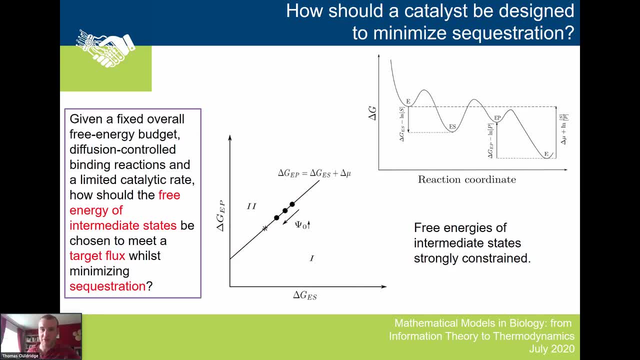 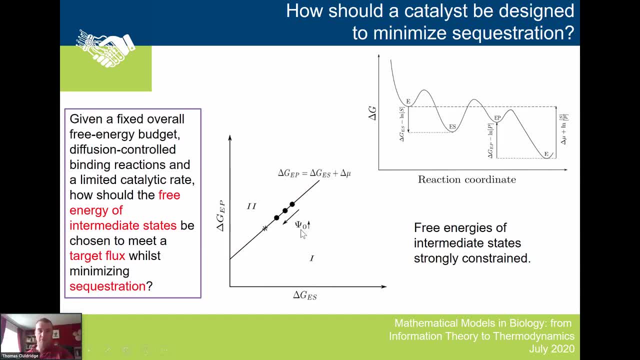 a certain flux with this And that's what this psi is. Don't need to worry too much. But if I'm targeting a certain flux, then I reach some point on this line. All of my solutions are on this line, which is a constant offset between the energy of the product bound. 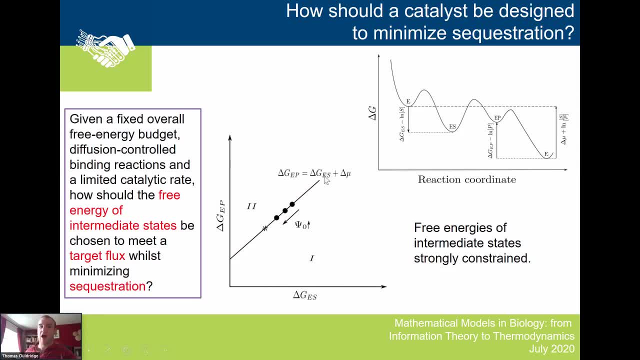 state and the energy of the substrate bound state, And the offset between those states is exactly this intrinsic free energy difference between the substrate and the product. So there are lots of things you can delve into about this result and exactly how we get to. it's quite interesting, but the real physics that's coming. 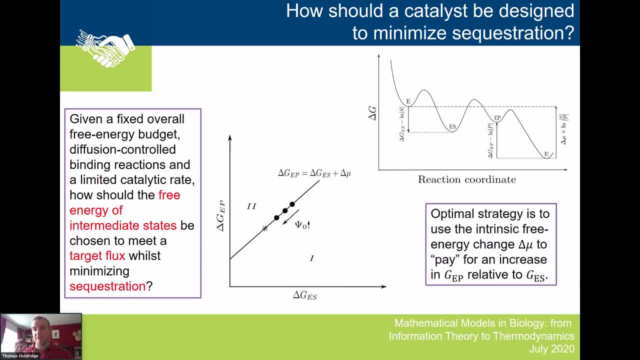 out of here. it's saying: the optimal strategy is to take this intrinsic free energy change that you get from converting your substrate into the product and use it to pay to make the product bound state Less stably bound than the substrate is. So what that means is that you can quickly 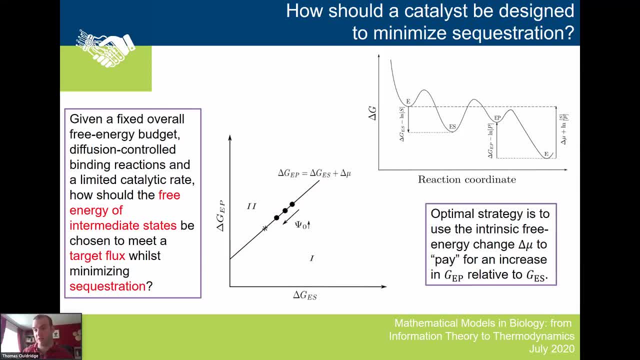 unbind your product once you've once you've had the reaction, But the, the, the, the really nice thing that comes out of of this admittedly very simple model is that it's exactly the, the overall intrinsic free energy drive that you should be using to do that, If you, if 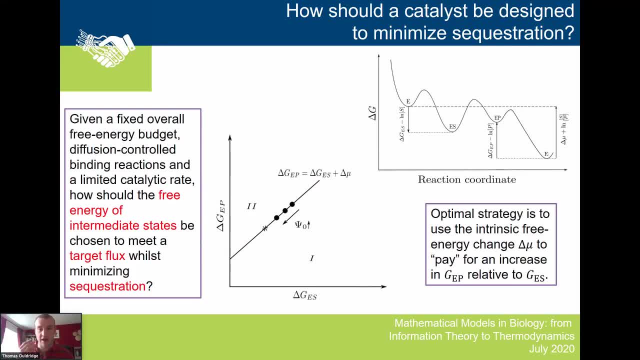 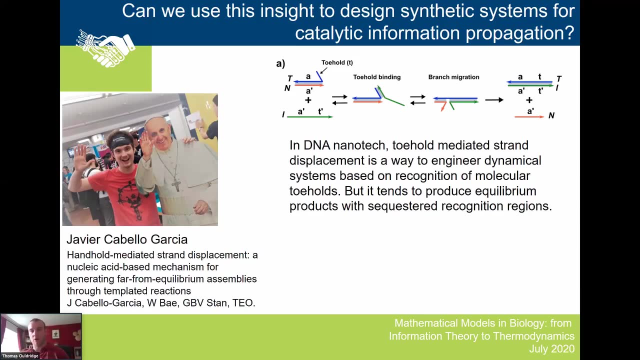 you want to design an optimal enzyme that minimizes sequestration. So what I'd like to do in the final part of my talk is talk about trying to use that insight to design a synthetic system for propagating information by a catalytic assembly on a template. 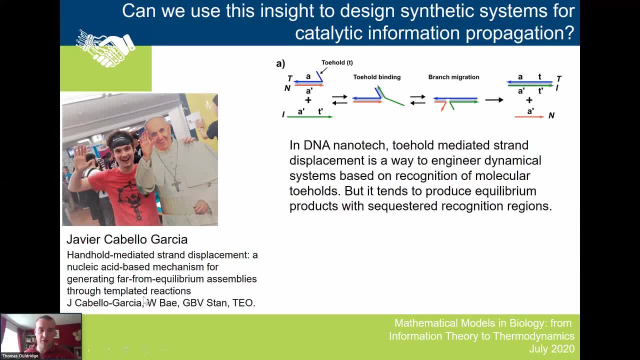 And so this is Javi's work and it's recently appeared on a bio archive, although I noticed that I actually cut off the The citation there. but yeah, it's on bio archive And there's a reaction again on my background is DNA, nanotechnology, And so this is based. 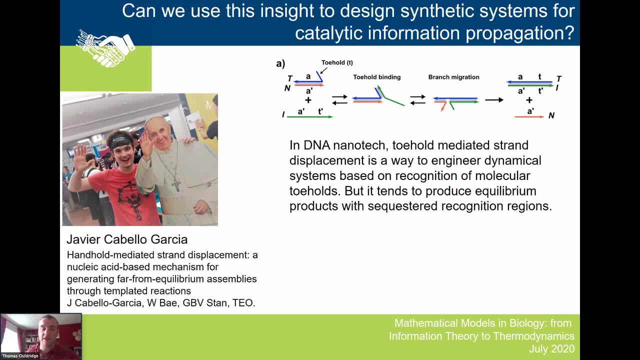 on DNA nanotechnology and in DNA nanotechnology, if you want to design a dynamic system where things are evolving over time, use a type of reaction called toehold mediated strand displacement. So you start off with a duplex labeled T and N, target and incumbent. 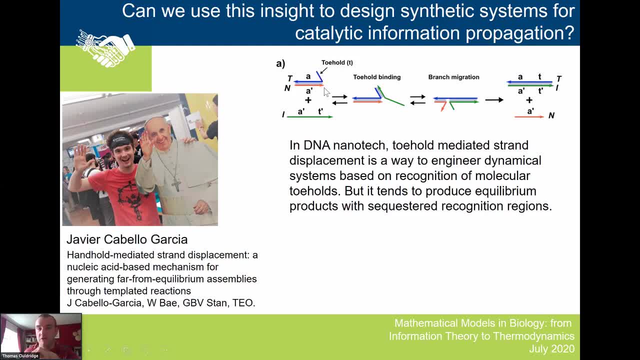 And the target has an overhanging toehold of base bases, which typically is about six bases long, And then you have an invader that's complimentary to the whole of the target and it, combined to the toehold, compete with the incumbent for binding to the target and then, basically, 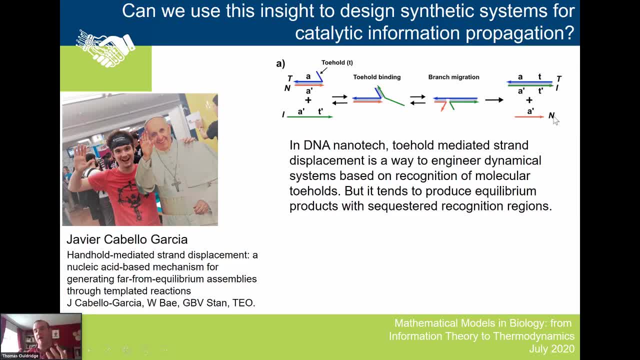 pull the target off the incumbent And by embedding this toehold mediated strand displacement reaction in more complicated contexts, you can actually build Sort of Turing, complete complicated reaction networks. I'm not going to go into the details here, but the but the. that's the essence. The important point here is that what you 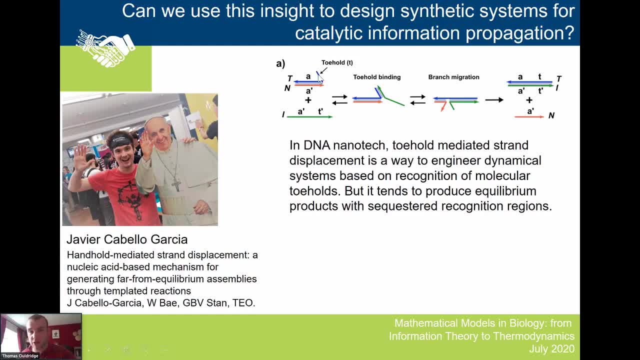 have is. is recognition based process right? You have, the toehold is providing the recognition for you, a bit like the way a template provides the recognition for the assembly of, of, of of these polymers in The molecular dogma, the central dogma of molecular biology, but the, in this case, at 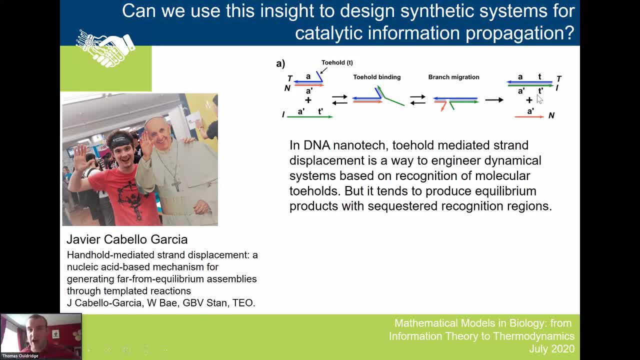 the toehold is here and the final bound domains are next to them, So they they're behaving very cooperatively. So, fundamentally, the recognition domain is going to be used up by this process. You're never going to be able to use toehold mediated strand displacement. 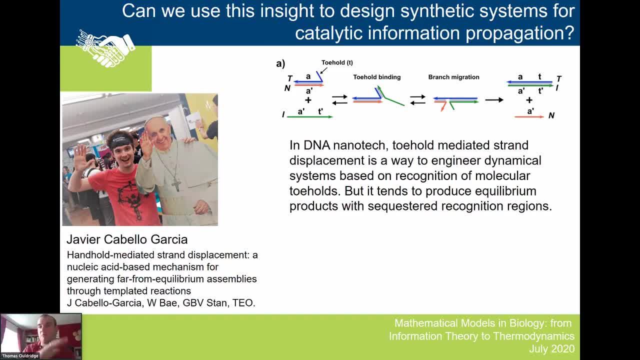 You're never going to be able to use toehold mediated strand displacement to perform a recognition interaction where that recognition interaction subsequently breaks- And if you remember, I was arguing that that's really what made copying of of, of polymers and so on, hard- is that you need to have a recognition interaction that later on in the 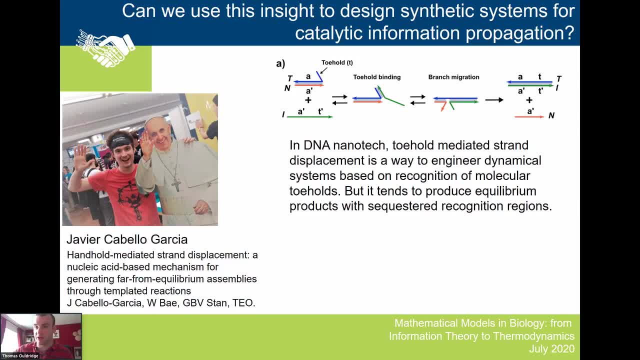 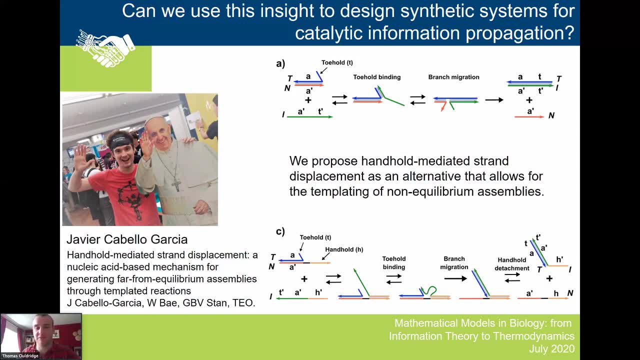 process breaks, so that you recover your product at the end of the process. Now, what have he is working on is an alternative scheme called handhold mediated strand displacement, And the idea here is that primarily, reactions are instead driven by a handhold in the incumbent. 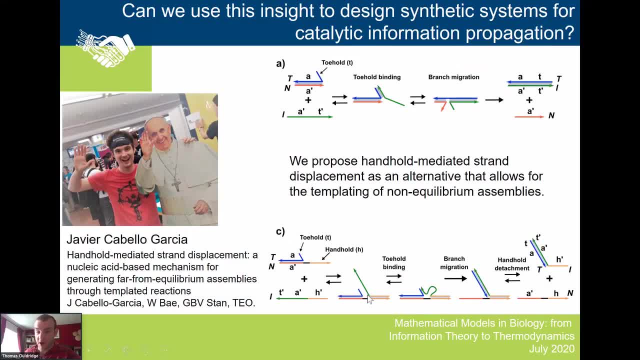 which is recognized by the invader. The invader binds to that handhold and then starts competing with the incumbent for binding to the target. So what's happening here? This is our product formation step. This is going from substrate to product And what's happening is the formation of the. 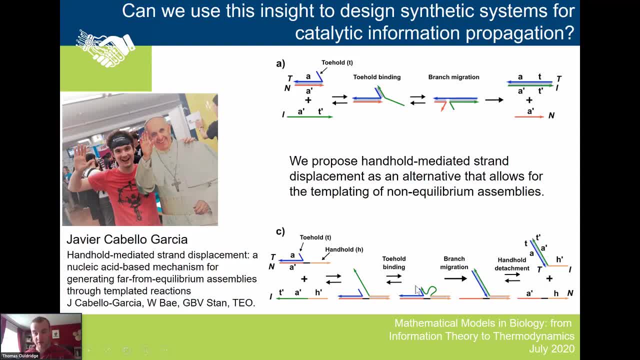 product is involving us ripping the toehold, the, the thing we want to bind to, off the, off the incumbent, off the template. So the, the formation reaction, the polymerization reaction, if you will, we using the free energy of the process to weaken our binding with the template, which is exactly the um uh. 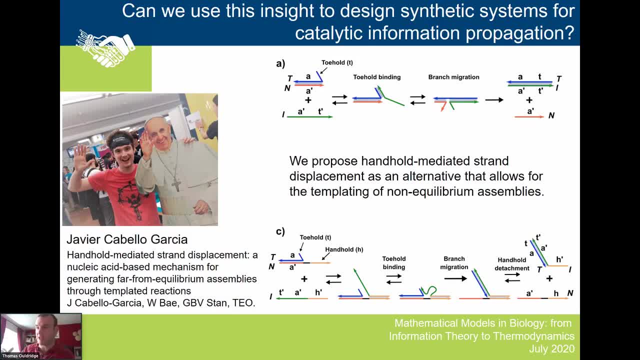 the insight that we got from Abishek's work. We should divert the free energy downhill free energy of the reaction And into weakening our binding to the, to, to the, to the substrate, uh, not so, uh, the template. 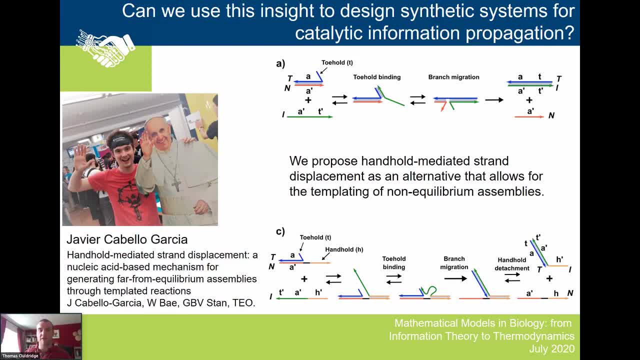 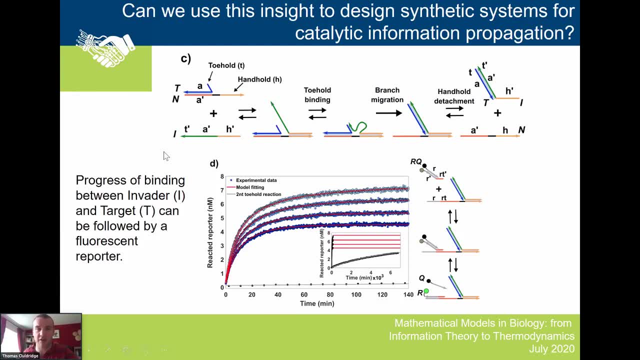 Um, okay, And so have. he has monitored, um the pro, he's been able to study a whole range of system designs, varying the toehold length and hold length, et cetera. Um, and what he's been able to do. you can basically monitor the formation of these products in in solution. 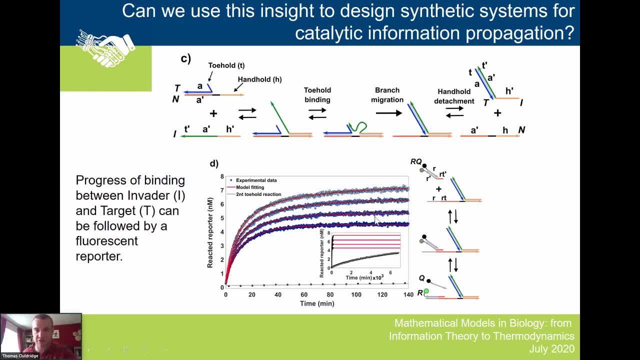 to this, Uh, and that's what. that's what I've plotted here. So this is just one particular system at different concentrations, and he's he's able to model them very precisely. So we feel I have a very good idea about what's going on. Um, and what he's been able to show is. 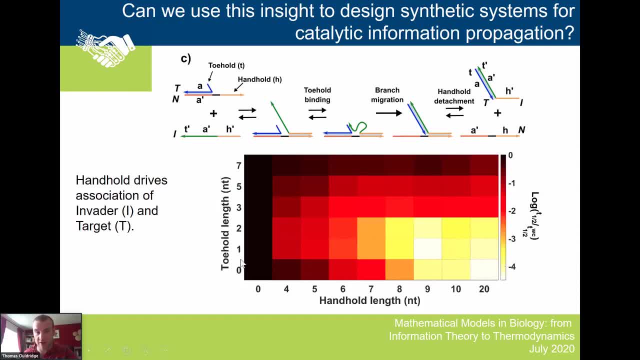 that as he makes his handhold longer for a given length of a small toehold here, he makes his reaction much, much faster. So this is the ratio of the half-life for a system for an invading strand with a handhold compared to one that doesn't have. So he's able to. 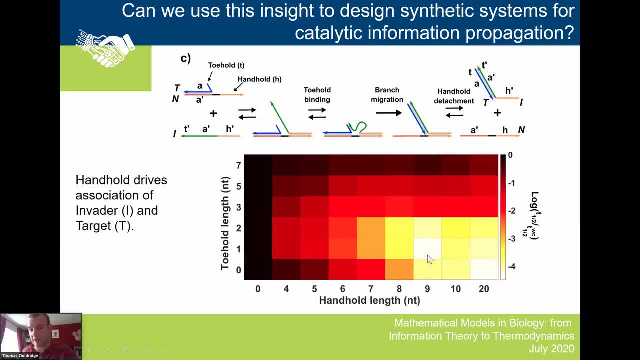 make the handhold, He's able to make the reaction for orders of magnitude faster than if he didn't have a handhold at all, for for for short lengths of these. So he's able to accelerate the reaction. He's able to demonstrate that this the formation of this blue green complex. 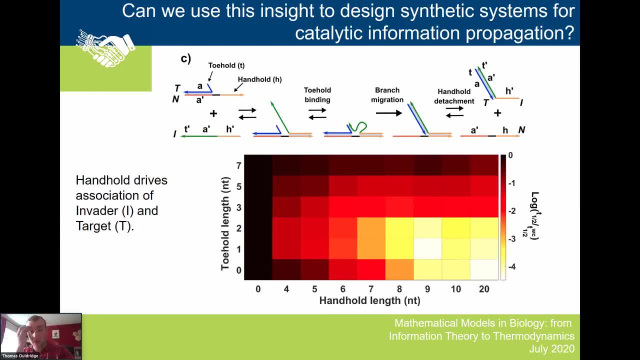 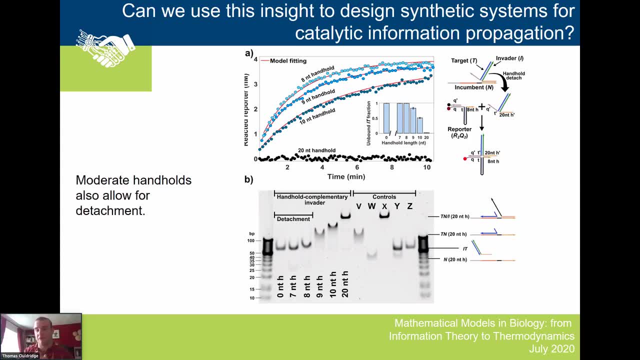 is, is faster. What we also need to do is demonstrate that um, actually Okay. Um, this recognition interaction can be transitory, can break after the product is formed. Um and uh. yes, let's just look at the top one of these two figures. Um, he has another fluorescent. 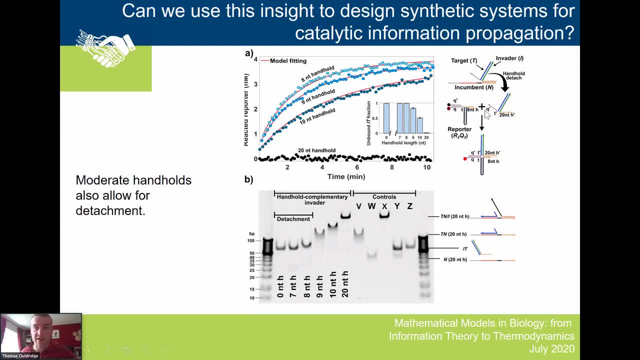 reporting device which this time, will only react if it sees a target and an invader. complex that is free and solution, rather than bound, still bound to the incumbent, And what he's able to show is that, if his handhold was really long, 20 nucleotides. 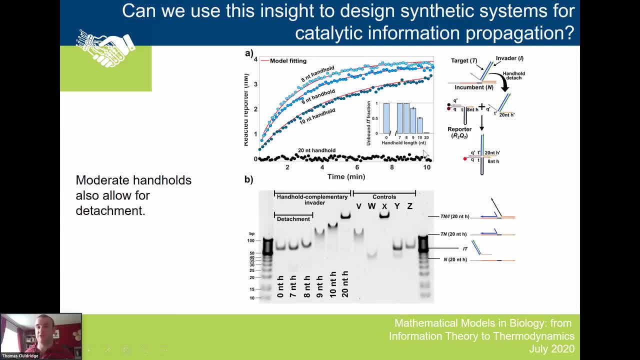 Okay, This reporter wasn't triggered because the thing never detaches. The handhold is too strong, The recognition interaction is too strong. However, the shorter recognition interactions, he sees release of the product. So he's able to use the handhold to template the formation. 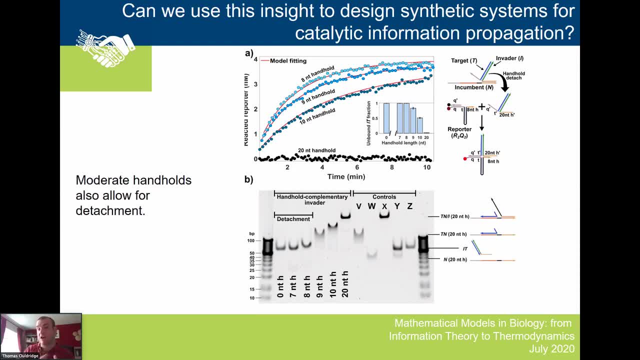 of the product, but then the handhold breaks and the product is released and is able to have an independent existence from the- uh, the incumbent. So the final thing he did was then to say: okay, can I use that to generate a non-equilibrium? 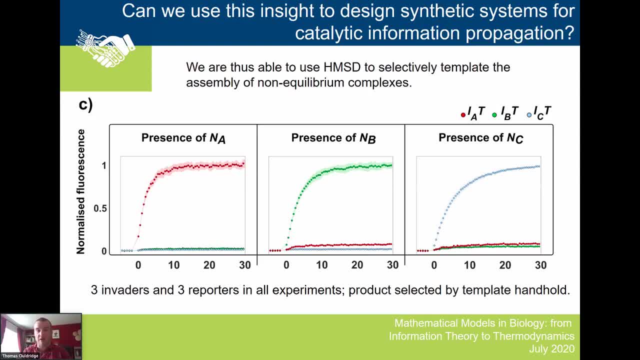 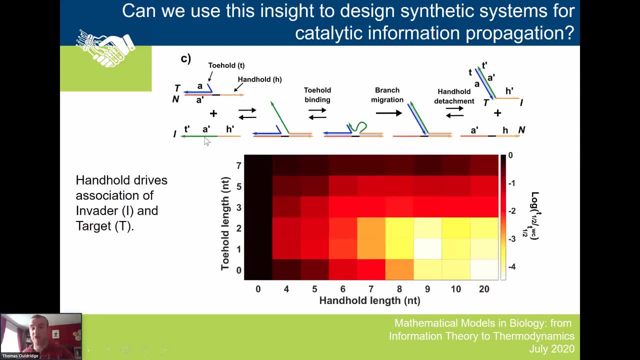 ensemble of complexes. So he started out with um, all three invaders, So all three of these strands, or three different types of these strands, or with a different handhold and uh reporters for each of those strands, And he puts in templates for one handhold or another. 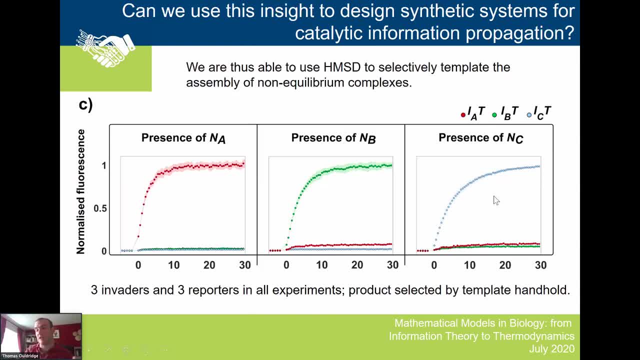 handhold or another one, And he was able to see essentially perfect formation of the desired complex. And what? what I want to emphasize about these results is that the duplex that's forming in the end is equal stability, whether it's the first type of 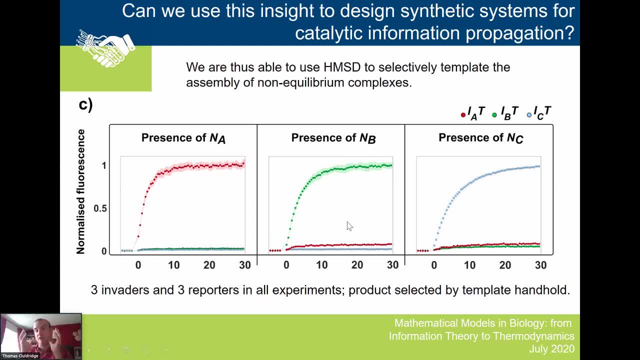 invader, the second type of invader or the third type. they're not distinguished by their chemical free energy. They're equally stable. They're just driven by this um transitory templates. So we really have taken like the first step towards generating a non-equilibrium. 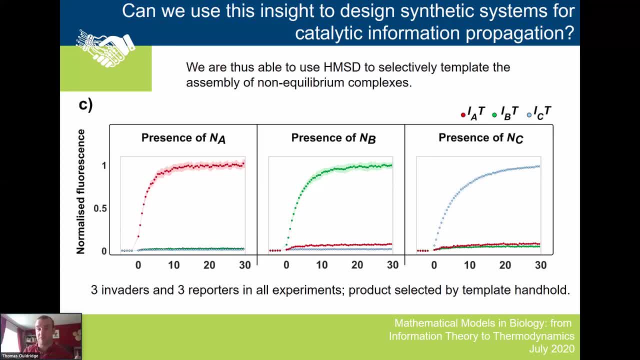 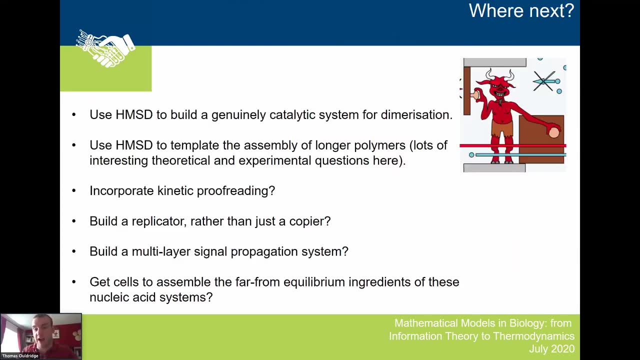 ensemble of outputs which does, I argued before, is, at the very basic level, what the copying of a, a polymer, is doing in biology. Okay, So that's basically it. where we'd like to go next is to is to really use this reaction to build a genuine, genuinely catalytic system. 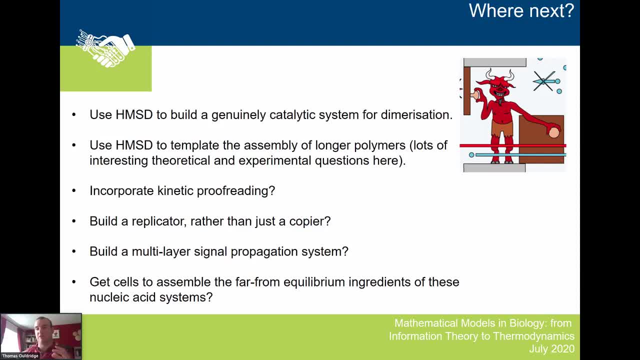 for dimerization. So so here We kind of the second half of the process, but we didn't do the initial recognition, uh, of the first half of the dimer, And then we'd like to go on to longer templates, So can. 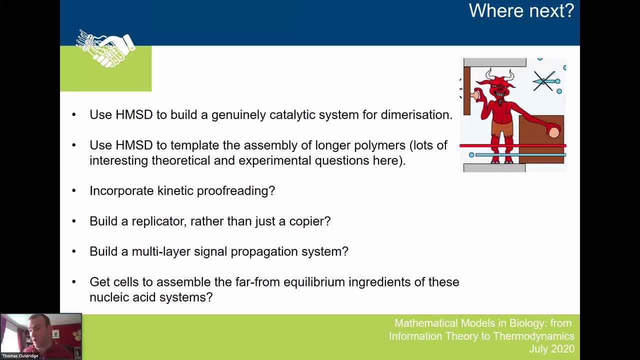 we really build things that copy information in a sequence of length- three, four, five, six and so on, And then there's a whole host of other interesting questions we can ask, Okay. So thanks to all of you for listening, Um, thanks to people in my group at Imperial. 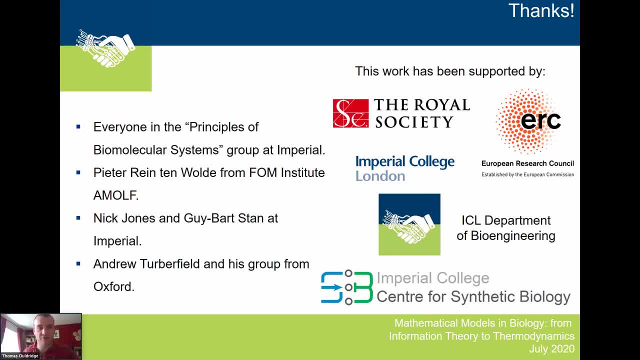 Peter Ryan. Um, Thank you very much, Thomas, for a very stimulating interesting talk. Um, we have approximately, by the schedule, we have approximately 15 minutes for questions, but what's after that is is just a break. So, uh, we can, we can, uh keep uh questions open for 20, 25 minutes. 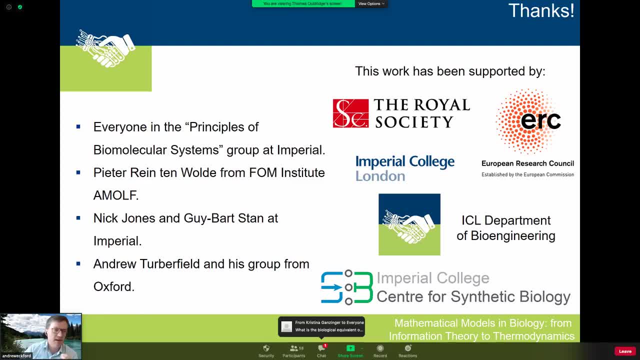 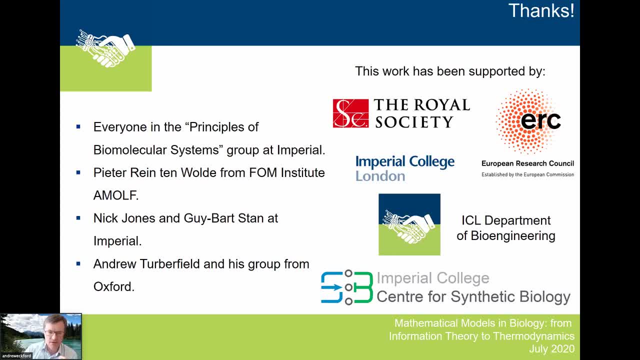 talks has been to um uh, to simply allow people to ask questions without, without my intervention. So, uh, please feel free to to unmute and um uh and ask your question. I see two questions just came up. uh on the uh on the screen. Perhaps Christina can go. 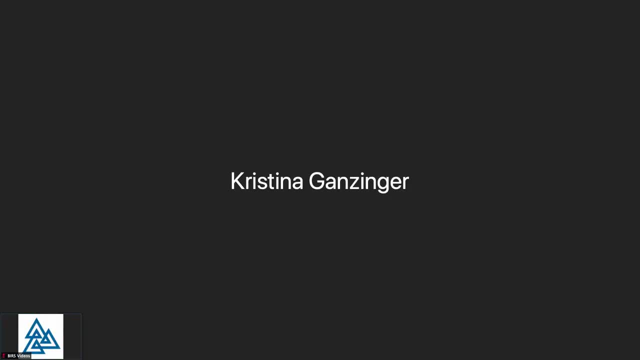 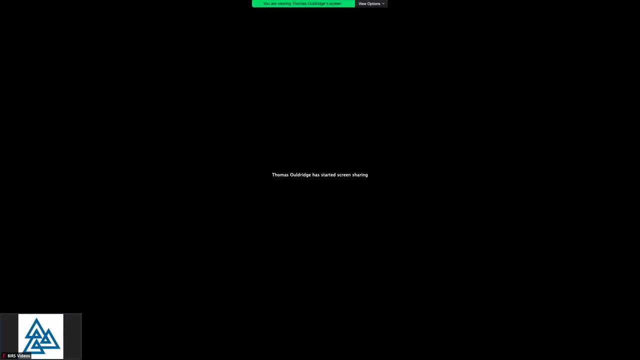 first. Yes, Just Okay. So, um, I'm going to, I'm going to go first. Okay, Start up my video. Yes, While you're getting ready, Christina, let me just say if you would prefer, if anyone, 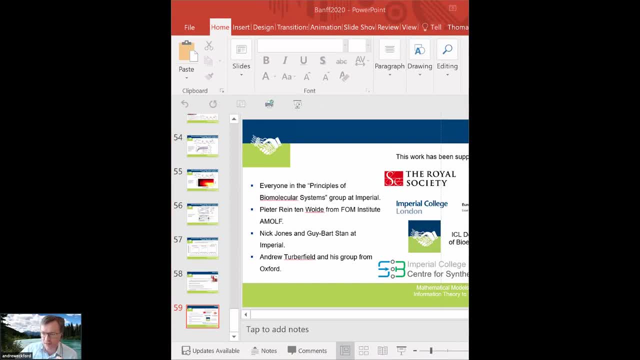 would prefer me to uh to ask the question on your behalf. just type it in the chat window and and ask and make a statement to that effect. Yeah, no problem. So I? I'm just wondering for the ModelDNA system that you were showing. 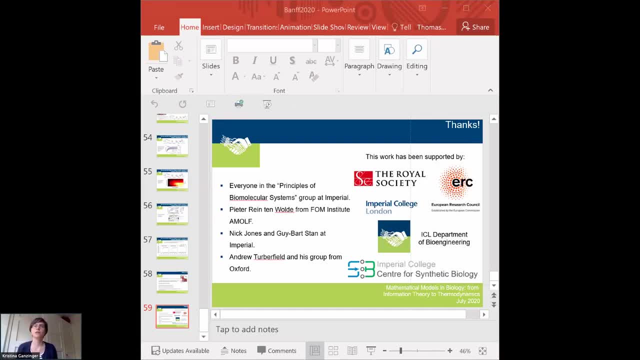 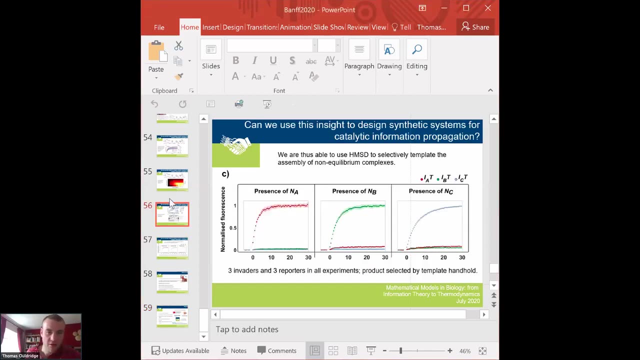 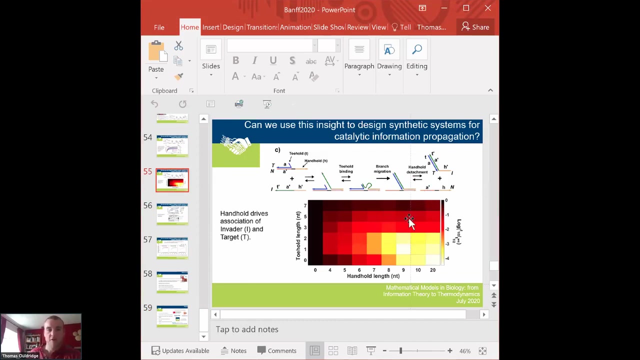 at the end what the equivalent of the invader is for, for um, for the biological system of RNA synthesis in transcription. Okay, so so, yes, it's a very important question. so, effectively, if I go back to um, if we go, if I go back uh to here, yeah, this will do so, um. 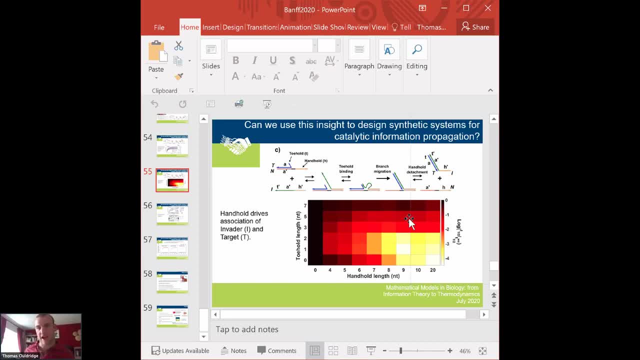 we are using whole strands of DNA to stand for one information bearing unit, so um, 10 to 20 nucleotides is our. is our one information bearing unit, as opposed to one nucleotide in or three in the case of um translation, but for transcription, one nucleotide. 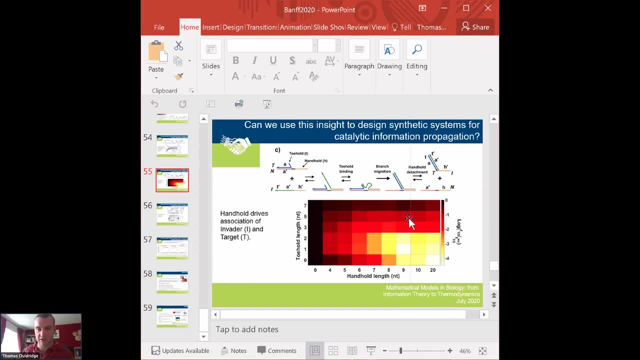 so the invader would be interpreted as the next um nucleotide that's being added to the process, and what we want to do eventually is build something that looks a bit like when you have RNA polymerase right going along a chain. we want to do it without 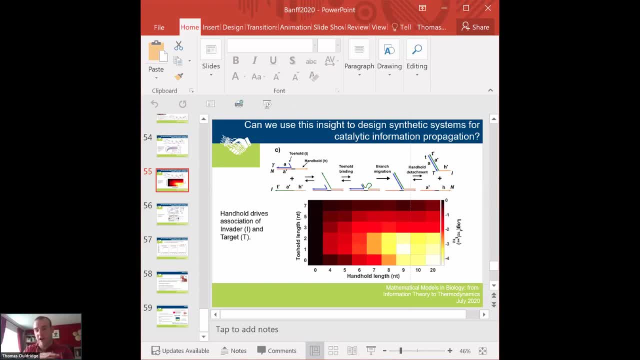 an RNA polymerase. but what? what you have is you have the DNA duplex, right, and then you have a growing single strand of RNA coming off it which is only attached essentially by its leading edge to the template, right, yeah, yeah, that's correct, yeah, yeah. and so what? what we want to do is: 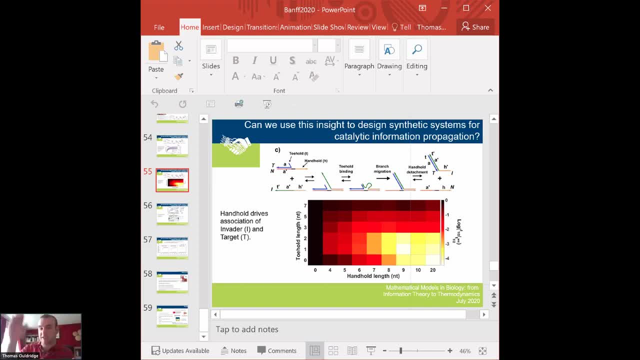 recreate that sort of thing. but each single strand coming in is the equivalent of one nucleotide and when the new single strand binds it rips the one behind it off the template and the whole thing takes a step forward. so you can see that you grow a longer and longer tail. 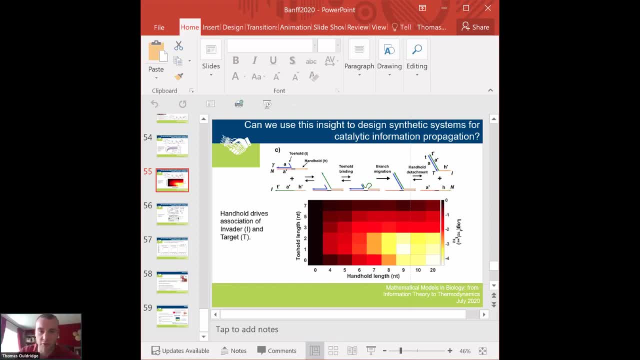 as the leading edge um moves forward. yeah, okay, yeah, that makes sense. now, just out of curiosity, is there a reason that you went for um, for modeling it like the entire piece of DNA as opposed to like shorter sequences or even single nucleotides? the reason we're using DNA is because we're able to rationally engineer interactions with DNA. 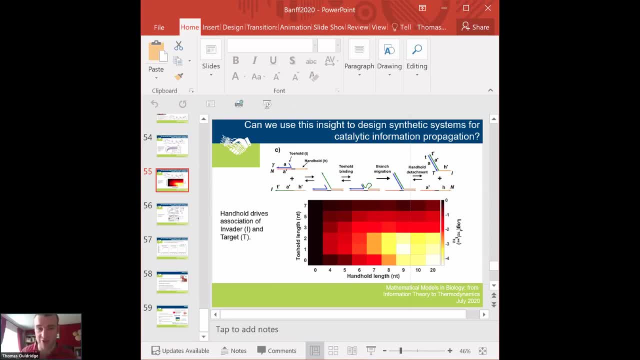 so we're able- I'm able to- and I am not any good at chemistry, right- I am able to- design things to interact with one thing and then interact slightly more strongly with another thing and then grab something else in a way that I just can't do, and I don't think even really good chemists can do with much smaller molecules. so obviously, 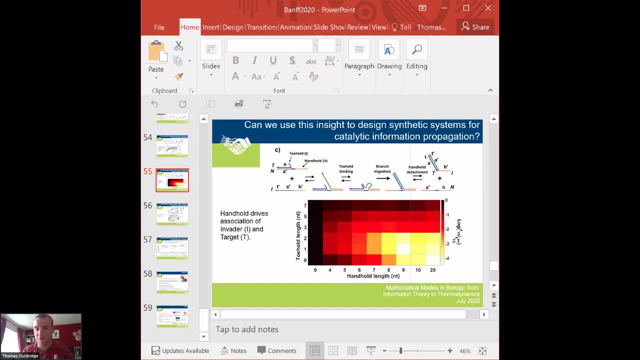 nature has found a way to do that, through a lot of trial and error, basically. but what? what working at the level of whole strands enables us to do is to rational design of these things? yeah, okay, but yeah, the fact, the fact that it's the, it happens to be, the genetic thing in cells is 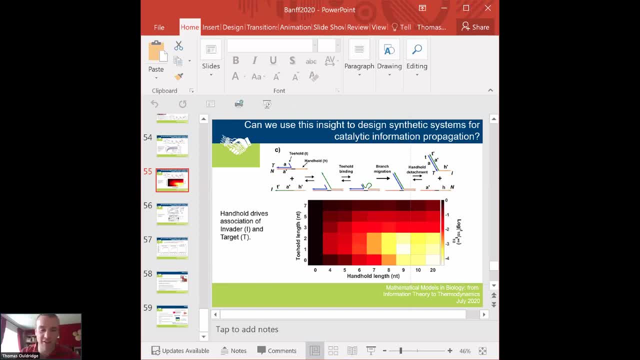 I wouldn't quite say coincidence, but it's, it's not. it's not what we're using it for, we're just using it as a selectively sticky molecule. so if you were able to give me another selectively sticky molecule, I'd be very happy. and what? what I want to do eventually is when we've really understood. 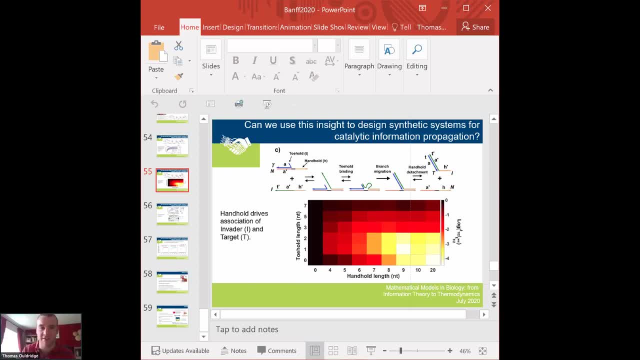 the, the constraints under which these systems operate is go to some good organic chemists and say, okay, this is what I need some molecules to do. can you, can you find someone to do that for me? you may cant do it. yes, easier to tinker and find out what you need at the level where, at the using whole dna strands. 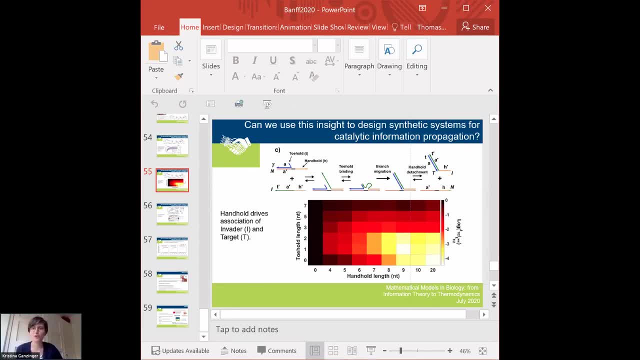 yeah, sure makes sense. maybe one last question, and then i'll leave the floor to someone else, and that's about the kinetic proofreading: whether you already have any ideas on how to implement this with the strand um displacement strategy that you are using. yes, so um. so, rakesh, who's? 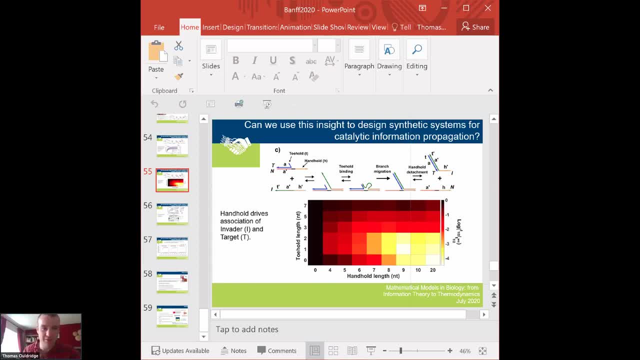 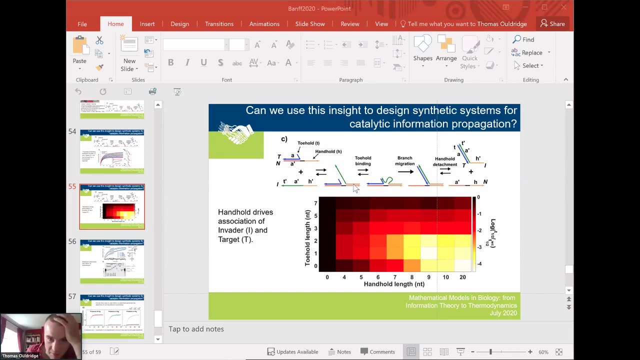 actually, i think on this call, that's his project at the moment- um and so the. the essential idea is: um, you can see my, you can see the talk. right, yeah, i can see the talk. yeah. so the essential idea is that the um, when this, when the, when the invader binds. 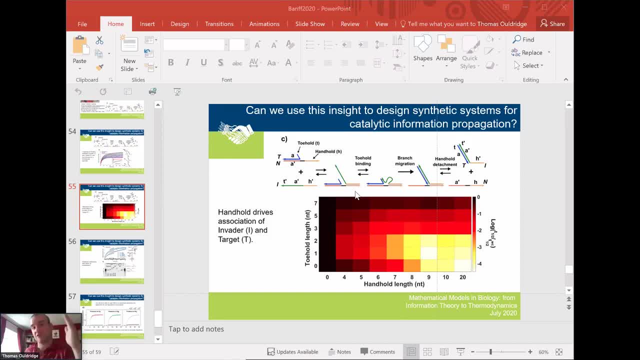 that it opens up a region that was previously hidden. so this invader would initially actually be um, um bound to a blocking strand, and it opens up a little toehold at the end and then that is. that gives the opportunity for a kind of like a proofreading molecule that's hanging around in. 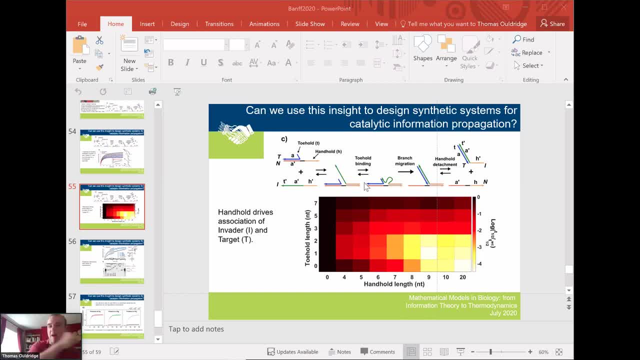 solution to come in and and and and rip it back off again, um, in a way that is dependent on how strongly it is initially bound to the template. so that gives you that's like rod rate: yeah, yeah, um and so yeah. the key point is: does that enable you to get discrimination both at the initial 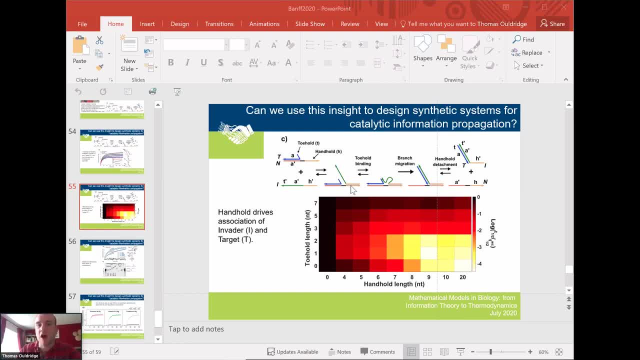 binding stage, which we should be able to do um fairly easily, but also getting the discrimination at that second stage that is sensitive to how strongly the thing is bound to the template that's uh, that's one of these key tinkering things that you have the opportunity to. 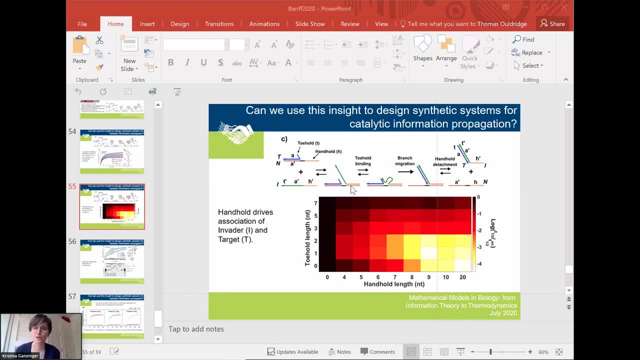 to do with dna nanotech? yeah, no, sounds like a really cool project. thanks, i have a question that's been sent to me privately and i've been asked to ask it. um, the question is: does sequestration give a strategy for binding the rna of a pathogen, such as, say, a virus? um well, 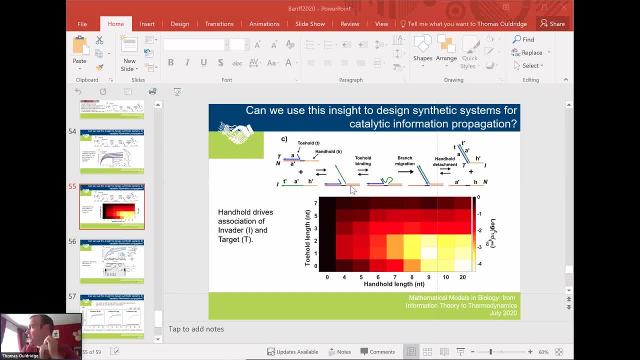 in the sense of: would you use sequestration during the rna's acting as a catalyst? um, i guess what you could do is design. if you were able to um, for example, screw up the translation process of some viral rna so that it didn't um got stuck. basically, maybe that would stop so many of your rna. 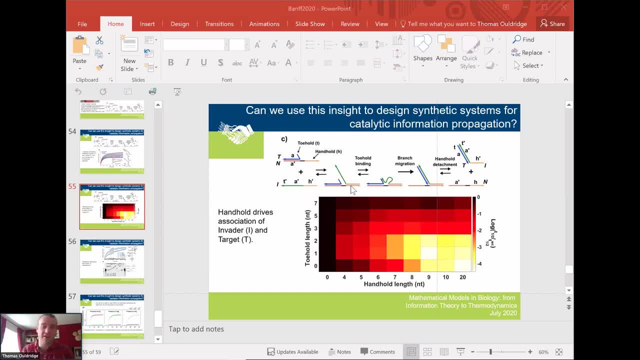 getting reproduced. i mean certainly binding to your rna strand and then, and then, and then doing something to it is a strategy that, um, that, uh, i mean, that's how crystal works, right? i think so. so it's just just using binding to to trigger some kind of downstream process that. 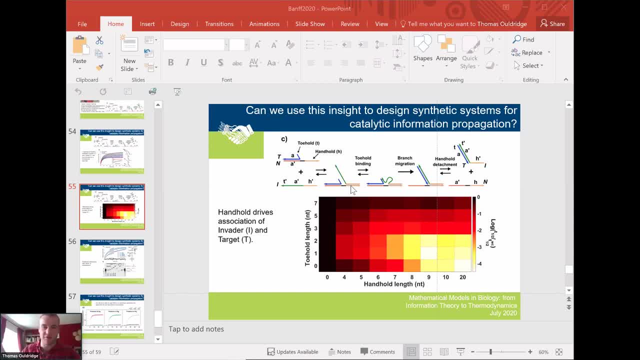 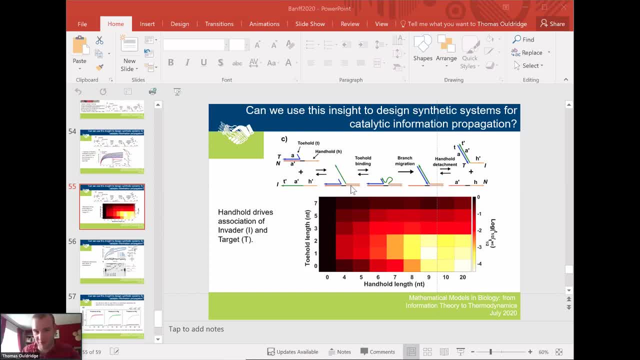 if anything does that it. i mean, it sounds like a more complicated way to to try and do the same thing. i don't know if that answers it. hey, uh, really nice talk. this is david savak. um, so your your idea about this challenge of catalysis being that you don't want to be? 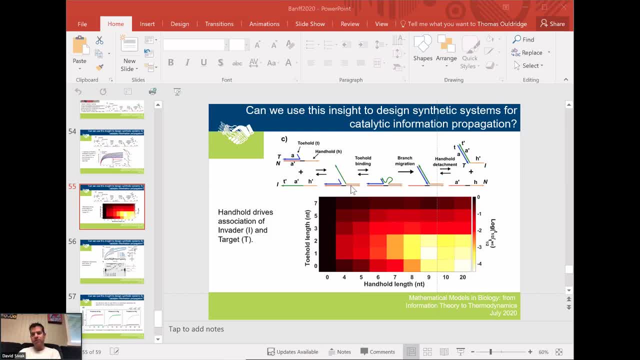 stuck to your product at the end of the day. i mean, i was thinking in terms of i don't know, sort of classic enzymology. you, you think about selectively binding the transition state rather than the product itself, and so is that. is that? how does that relate to the point? 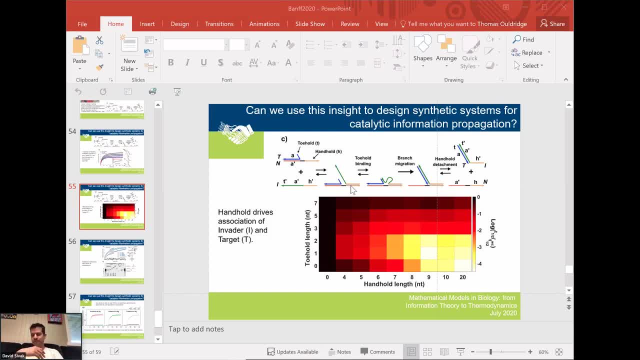 you're making here and are there like special challenges for these template mediated polymerization reactions that you want to? yes, i mean somehow, somehow in the discussion that i was given, we kind of assumed a certain thing about. we kind of assumed that the transition state was down to. 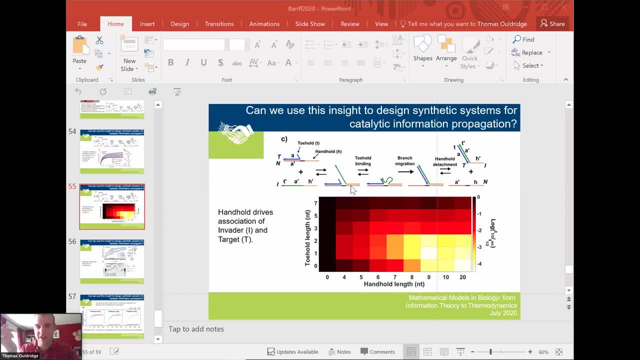 detail, chemistry and was was kind of fixed and all you could tune was the, the size of the wells on the other side, um, but fundamentally, if you, if you, you have to go through, the product is bound to the enzyme step and if you make it really really unstable, i, you really really don't want to. 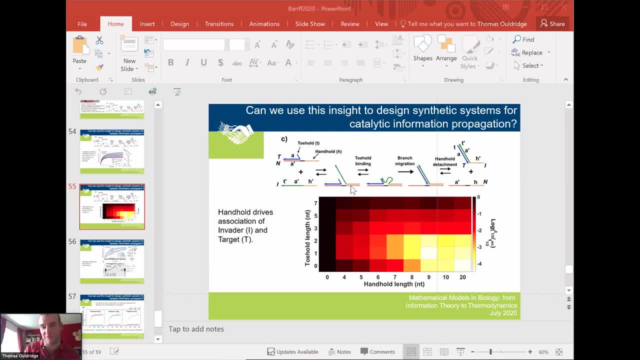 the product, then you're never going to get to that state in the first place. you make it too far uphill to to to go forwards. it will just stay in this, in the initial state. and if you make it too far downhill, then the product stays stuck to you and that's product inhibition and the the the answer. 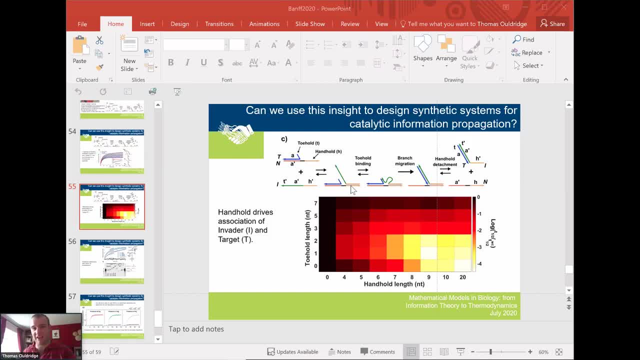 that abhishek got out was somehow quantifying exactly the fact that there's a sweet spot in the middle of both. um. but yeah, like in all cases, if you can make your transition state lower, you make it, you, you make it too far downhill and then the product stays stuck to you and that's. 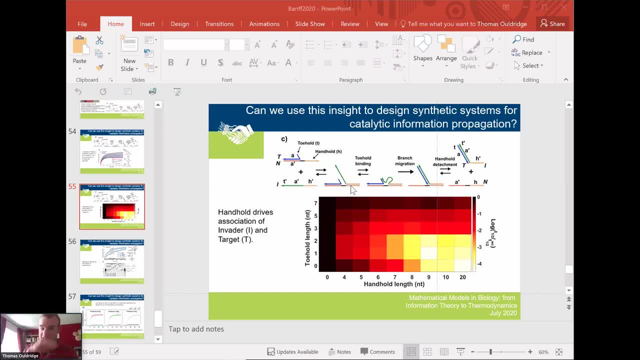 what makes your job easier. but even no matter how low your transition state is, that question of how strongly do you want to stay bound to the product is is still relevant. yeah, and maybe a related question, so, um so where did you use this theoretical knowledge in this? 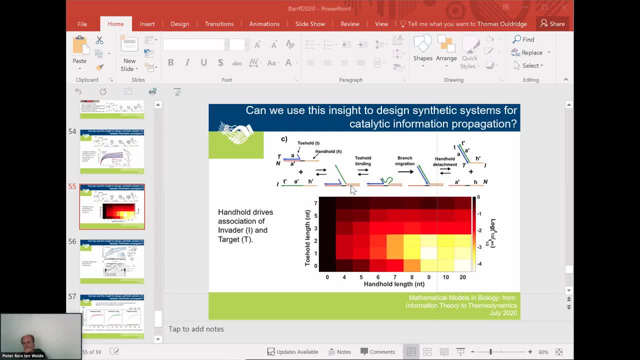 practical um experiment. it's just the central idea, which is the way that this mechanism works. is that one like you can think of, if you, if you can? you see my cursor at the moment? uh, i could, yes, i still yeah. so this, although we haven't quite got there,